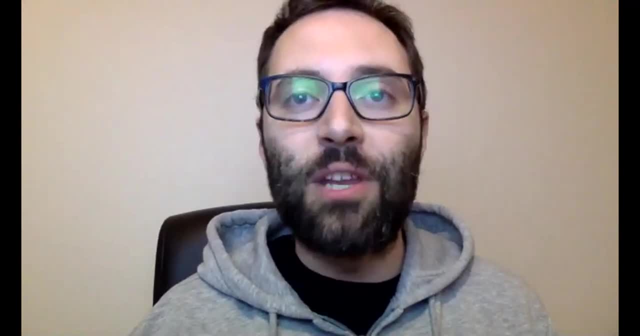 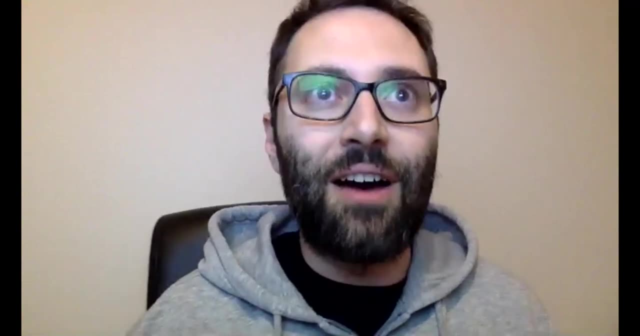 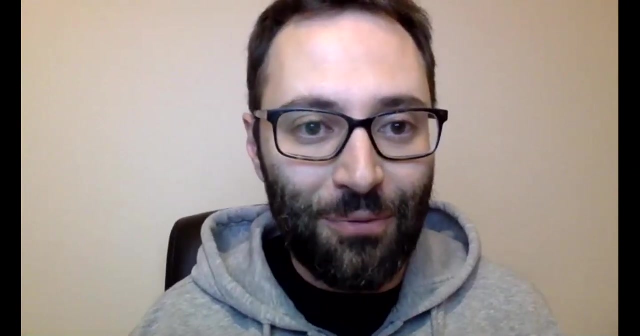 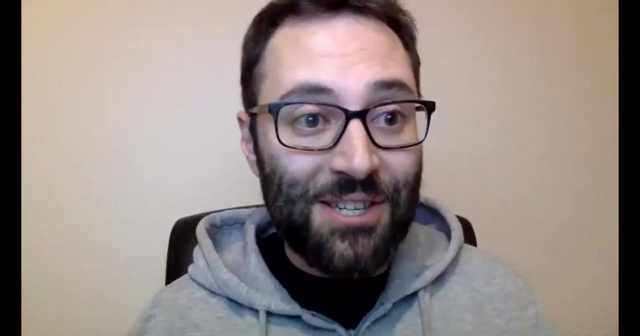 Robotics company and he will speak to us about their exciting new quadrupedal- a set of quadrupedal robots for real-world applications. Thanks a lot, Jing Yu, for coming and virtually speaking to our workshop. Thanks a lot. Please share your screen and we'll answer all the. 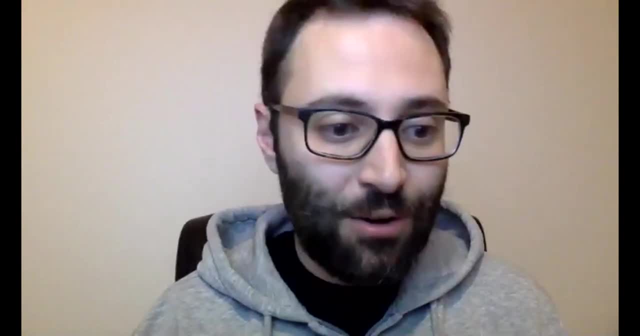 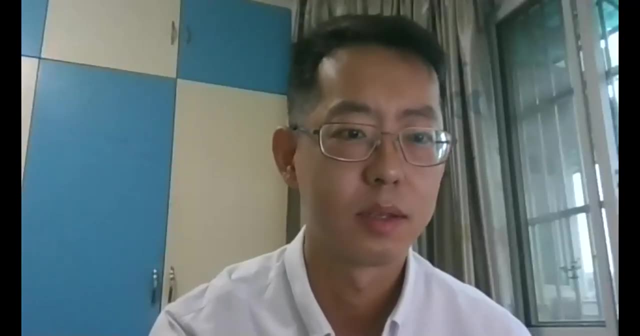 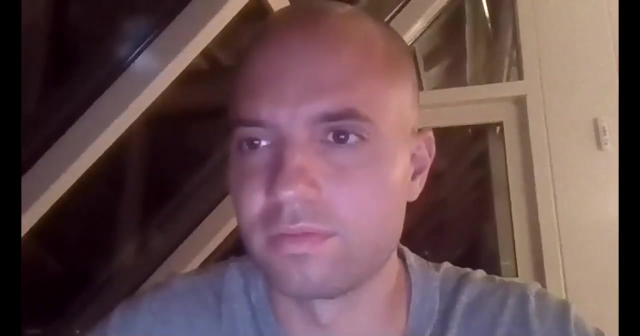 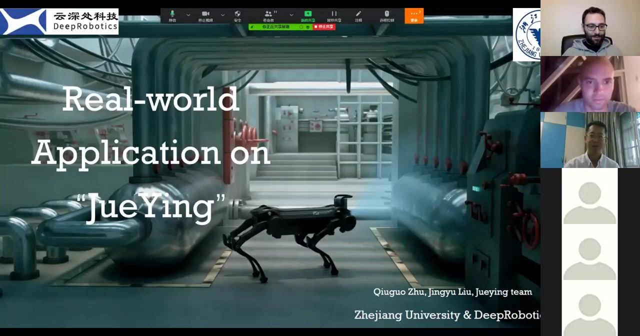 questions. You will be Able to answer all the questions in the end of the talk. Okay, Right, Hello everyone. Welcome to my talk today. My name is Liu Jing Yu from Deep Robotics. I am, Oh, hello, My name is Liu Jing Yu. I'm working in the robotics field. I work as a locomotion algorithm. 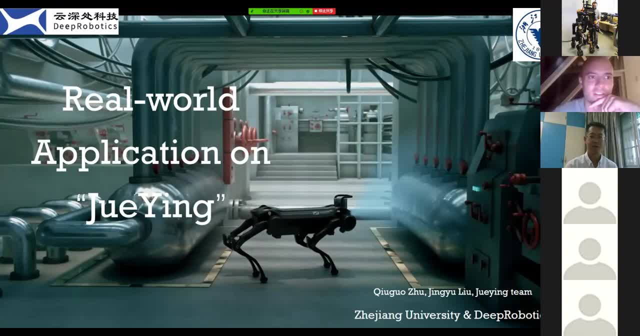 engineer in deep robotics, And I got my master's degree in Tei Wu Diamond, And my study was basically focused on the state estimation and control theory and application, And I'm here to speak on behalf of Dr Zhu Qioguo, who's the assistant professor at Zhejiang. 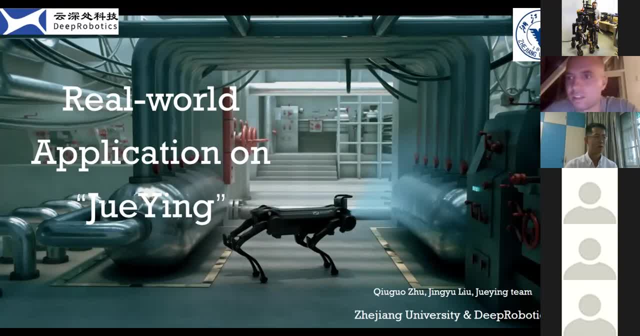 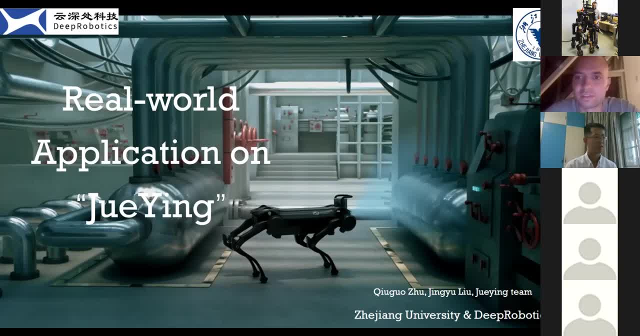 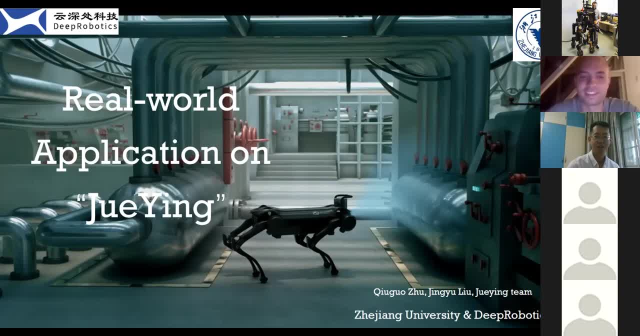 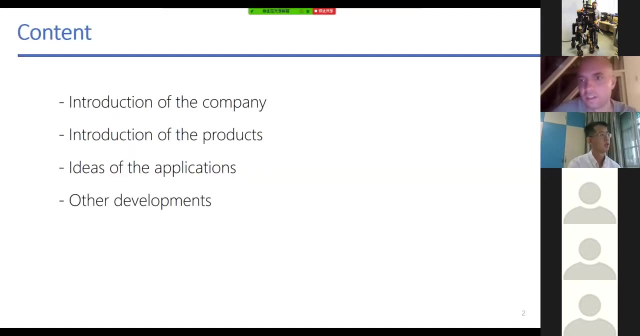 to host a meeting online. So let's get started. My talk today is real world applications on Jueying. It will be divided into four parts, which are: introduction of the company and the introduction of the products, the ideas of our applications and some other developments. 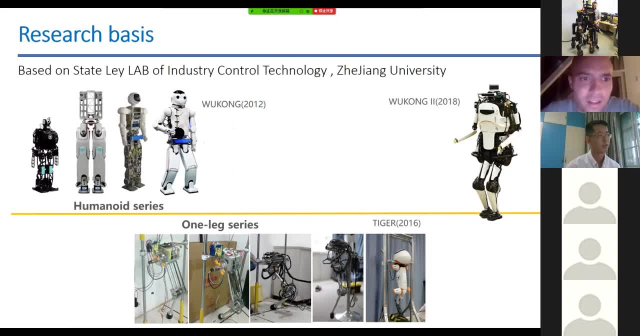 And our company is a startup company founded in 2017.. And earlier before that, Dr Zhu Qiuguo did his research on lab robots. that is based on the state key lab of the company, And Dr Zhu Qiuguo is an industrial control technology. 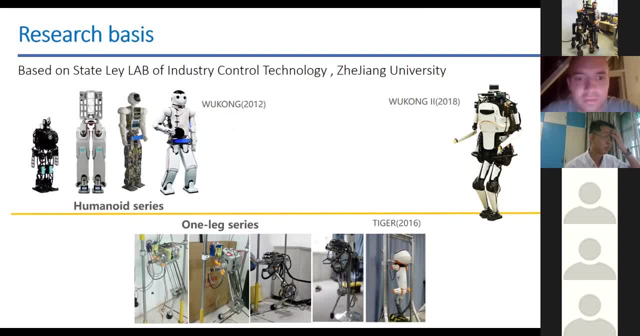 at the Jueying University And we can see in this picture there are two series of the robots has been developed. One is the one lab series And we all know that the one lab series is the basics of basics when you want to develop quadruped. 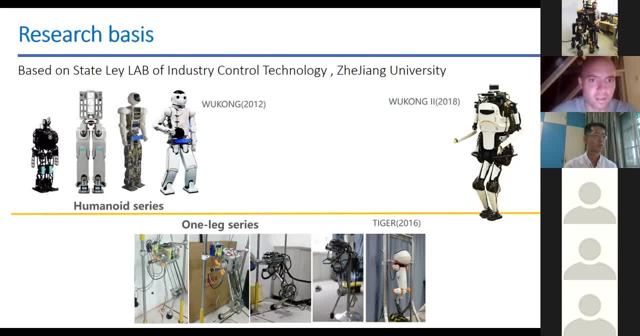 or humanoid series And you can verify your series and some other things in the one lab series And you can verify your series and some other things in the one lab series to do a lot of practice on it And I want to introduce the Wukong human lab series. 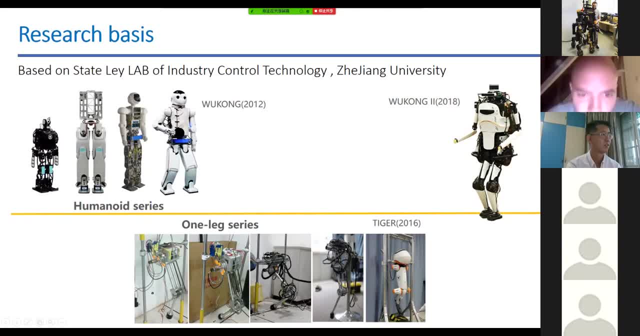 We can see the top left, the white one. He's holding a ping pong bat And it was the first robot that can playing ping pong with the people. It was in 2012.. It can also kick back a spin ball. It was amazing in that time. 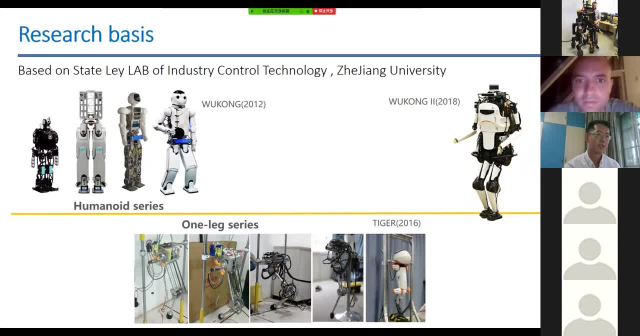 And in the right, in the top right, the two second generation of Wukong can run faster. It's around, it can run around like four kilograms per hour And it's also became more and more stable. It was also the first humanoid robot. 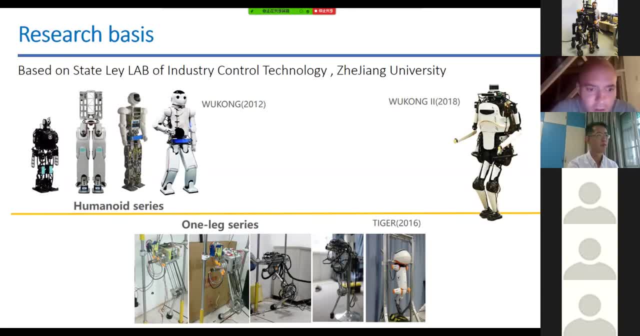 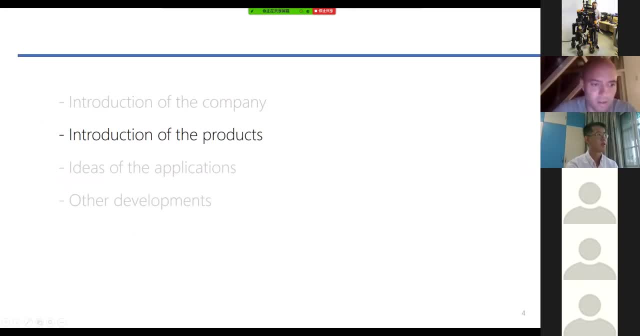 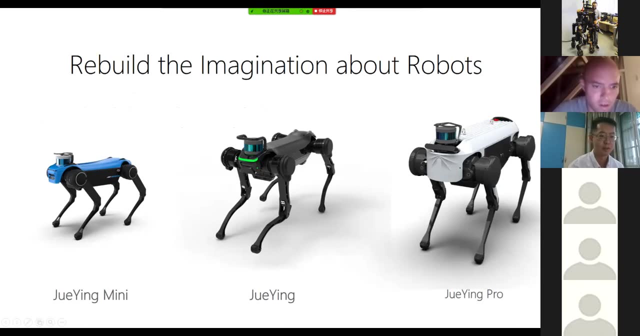 that can run this fast in China, million. And then let me introduce our products. Rebuild the imagination about robots are our slogans, of our company, And basically we have three different types of our product: The Drain Mini, Drain and Drain Pro. Here we go with the Drain Mini. 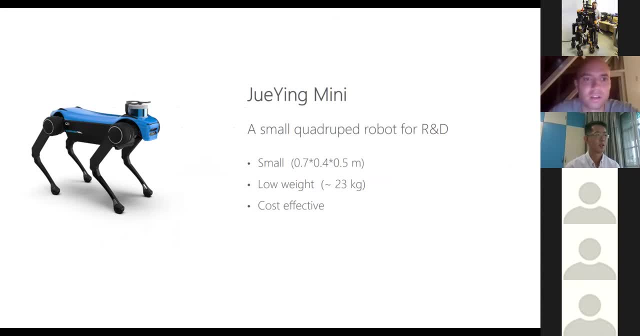 It's small and it has a low weight. This small dimensions are measured when it's standing And it's also. it's also cost effective And we believe that this small part of the robot can be very good for the research and the development. 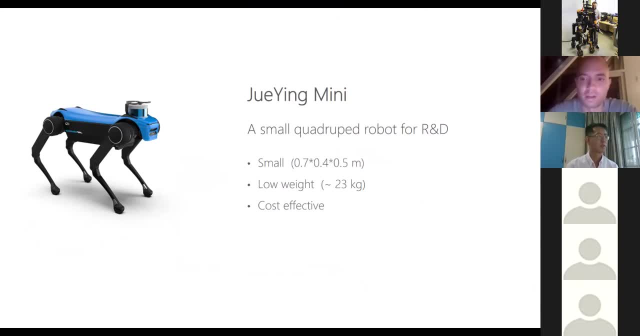 because it's cheap and it's all equipped with this lidar and the cameras can all be option equipped with this sensors And you can verify your control theory of the locomotion. or you want to do some deep learning on it or you want to do some slam. 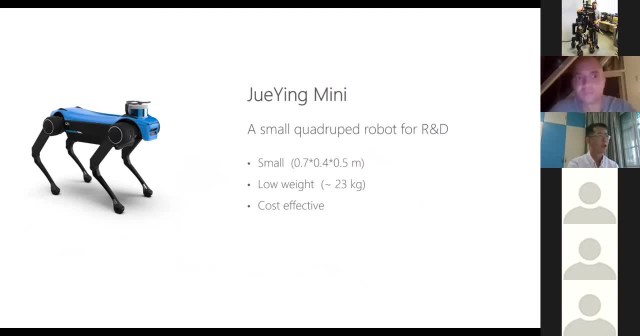 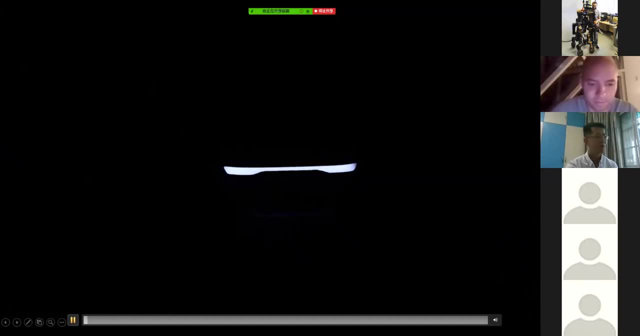 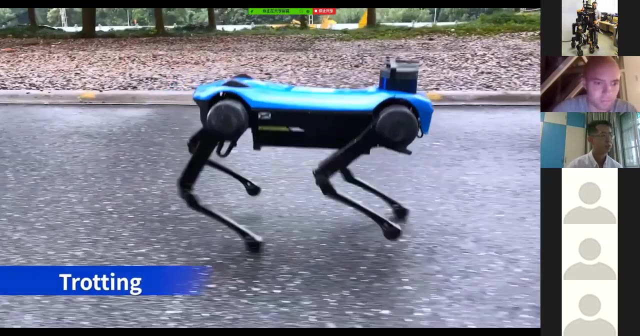 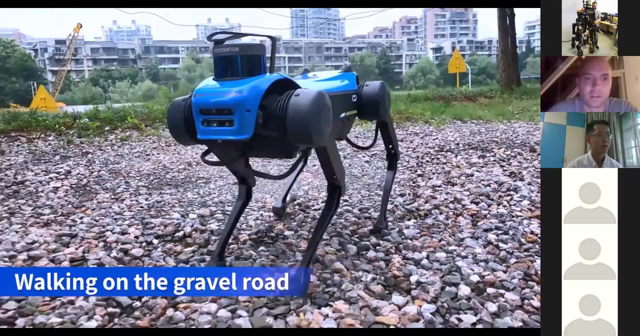 or algorithm on it. It can all be done. And let's see a video about the Drain Mini. It can walk and running. try running with a full, flat face. and also bonding on the gravel roads- not a big deal. Bonding on the gravel road is not a big deal. 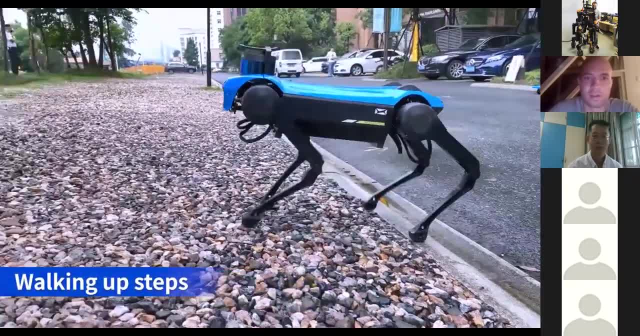 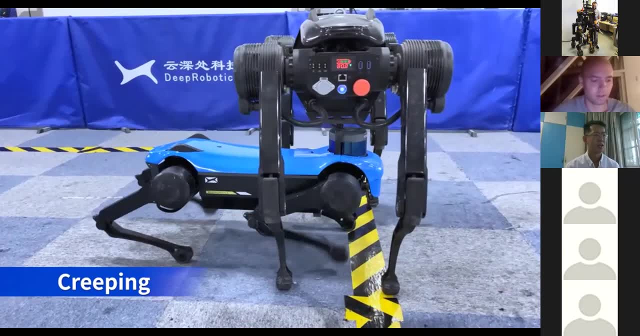 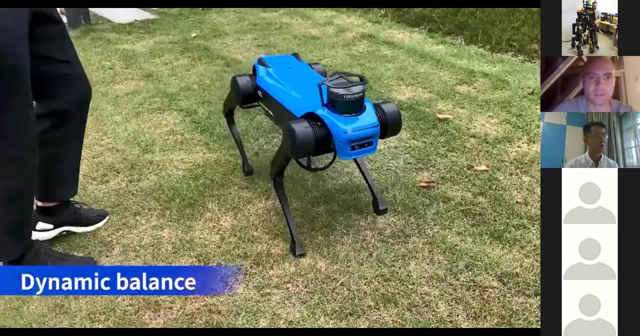 And the up steps and down steps is also not a big deal And because thanks to his small size can go very narrow spaces like this, for example in the industrial site pipe or something else. it can also keep balance after a disturbance and can do the autonomous navigation. 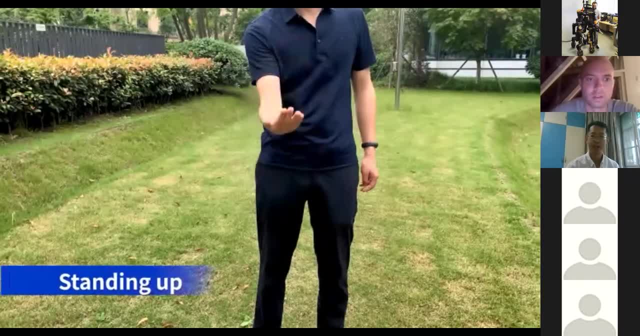 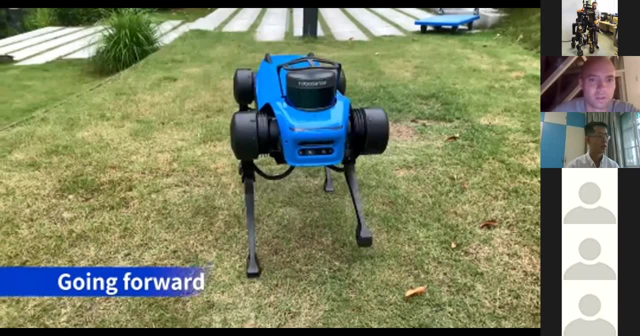 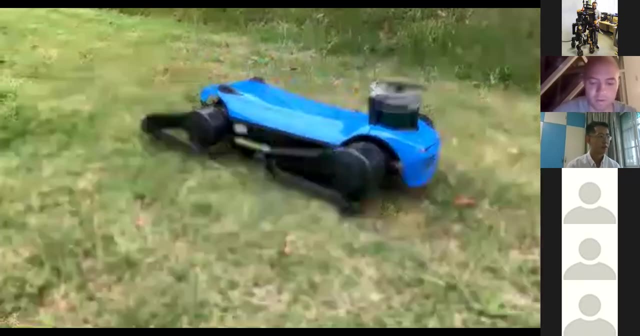 And the front two cameras can recognize the balance. It can also recognize the human body gesture as a specific orders and react with the different movements, like going forward and back forward and get down, And when he fell down can also get up by himself. 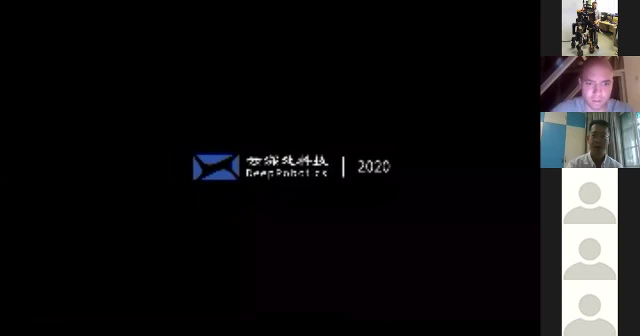 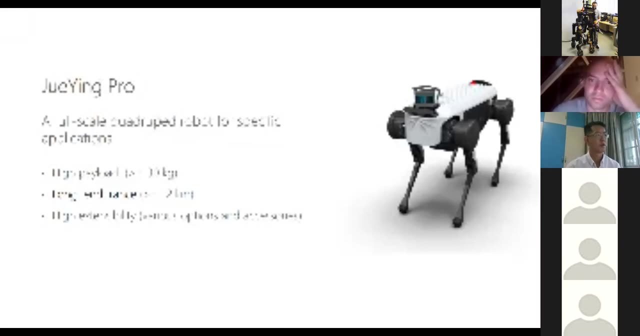 That's our Drain Mini, the smallest robot of ours. And here we go with our Drain Pro. It's a full-scale carburetor robot for specific applications. Specific applications we mean you can you have to add a lot of accessories on it. 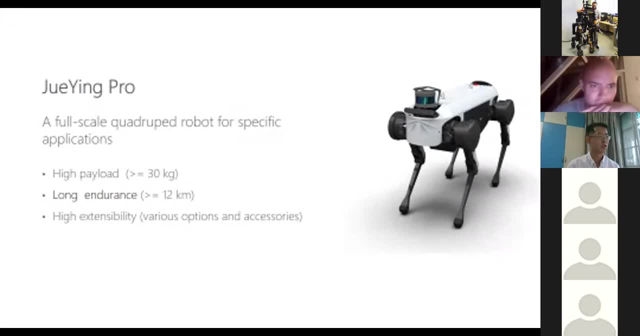 Thanks to its high torque motors on the joint. the payload of this robot can be more than 30 kilograms, And it can. it also has a very long endurance. We have tested it. It can work more than 12 kilograms without no parts at all. 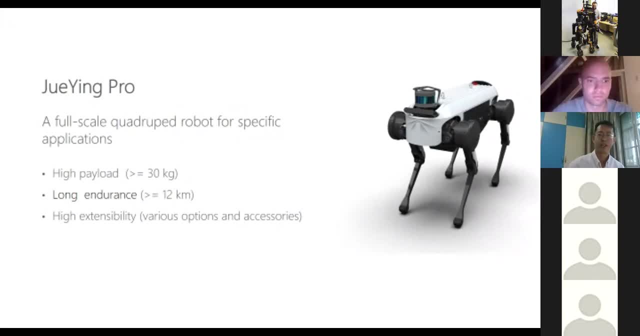 And if you want to add some like a robot arm or a professional camera pen, it's gonna be very heavy, So you can put it on the top of this type of robot. And let me introduce our the project that we are under development. 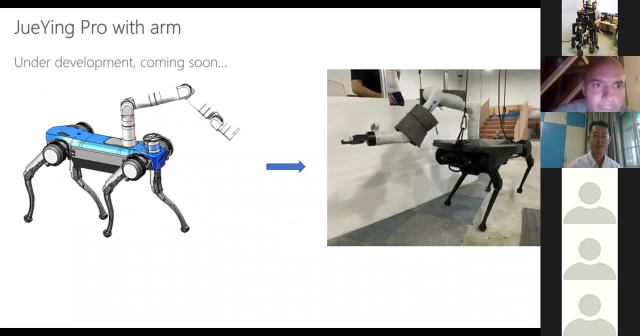 The robot Drain Pro with an arm And as far as I know it's gonna be the first robot with an arm on it in China media And theoretically the one arm- one robot arm- weights like six to eight kilograms, So theoretically we can add two arms on it. 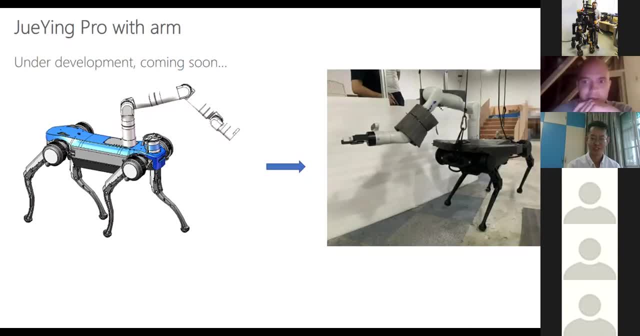 but it's gonna be very not so good looking. So theoretically we can add two arms on it, but it's gonna be very not so good looking. So theoretically we can add two arms on it, but it's gonna be very not so good looking. 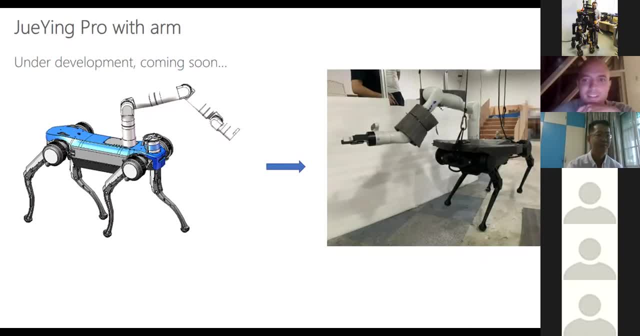 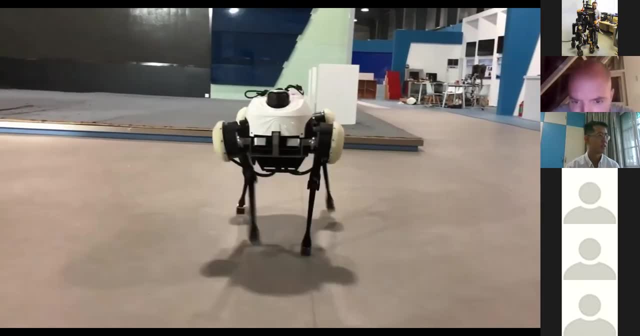 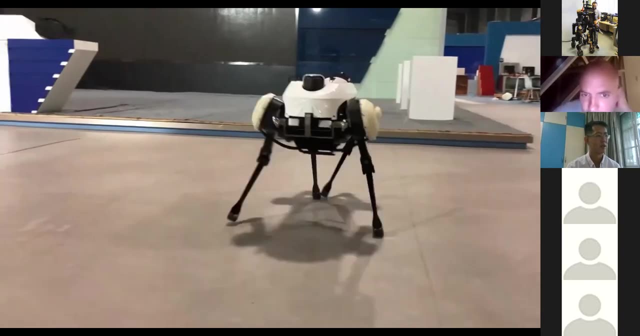 So theoretically we can add two arms on it, but it's gonna be very not so good looking. Let's see some videos of our past. It was in 2017.. The early type of our quadruped robot. It can step aside. 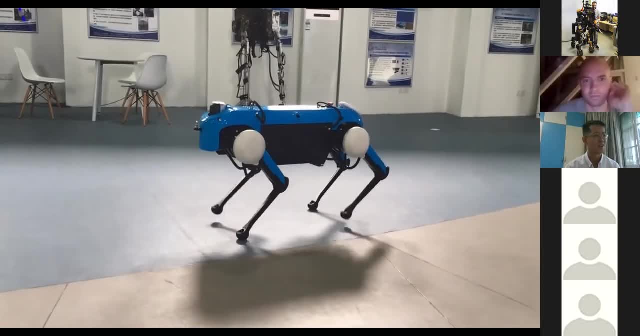 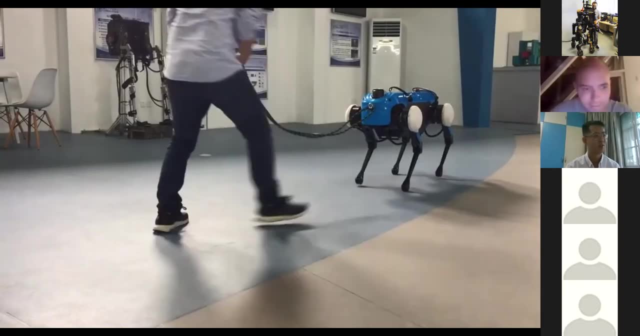 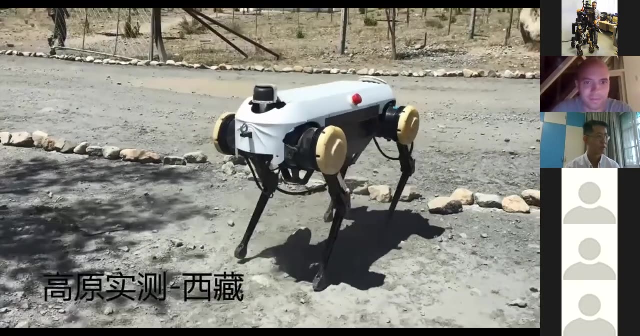 and we were allowed to kick it in that time, not right now- And it can keep balance after kick, after drag also, And it was in Tibet in very high altitude, And it was in Tibet in very high altitude After he stepped on a log. 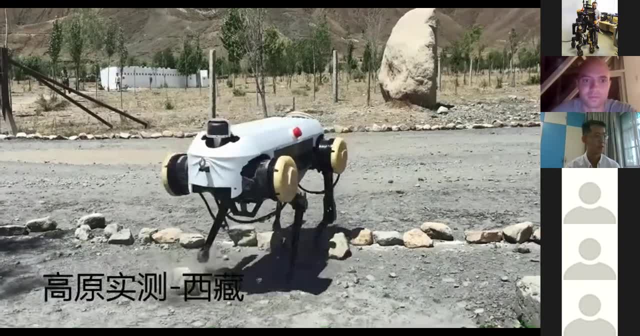 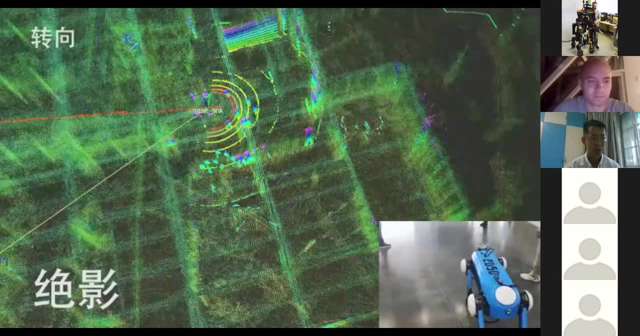 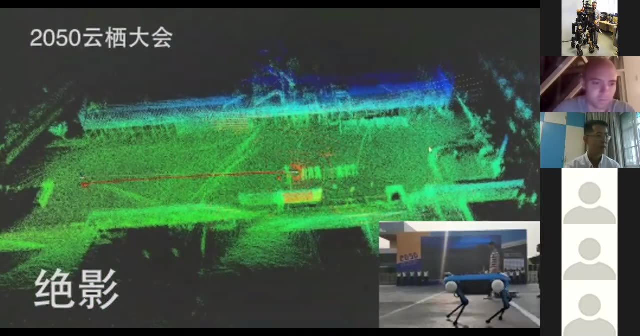 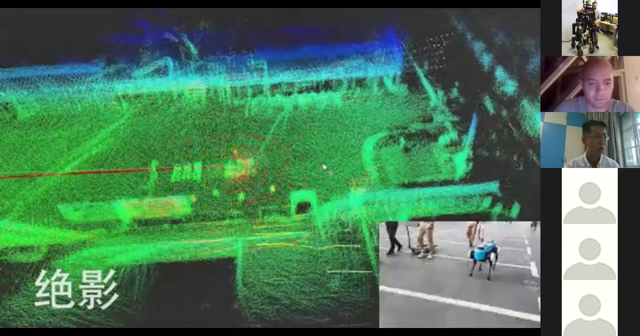 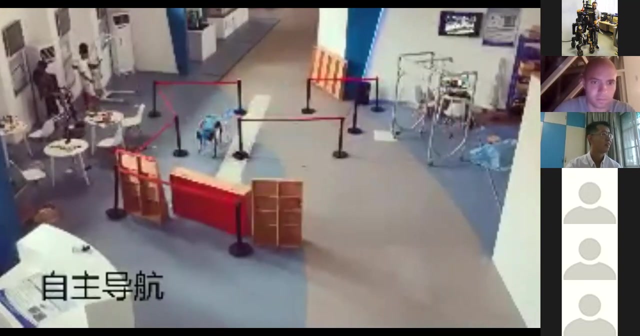 it got some slippery but it can balance itself very quickly And it also can do the navigations on both indoor and outdoors. This was outdoors And this basically all the old videos. This our first generation of the navigation. These videos are all speed up. 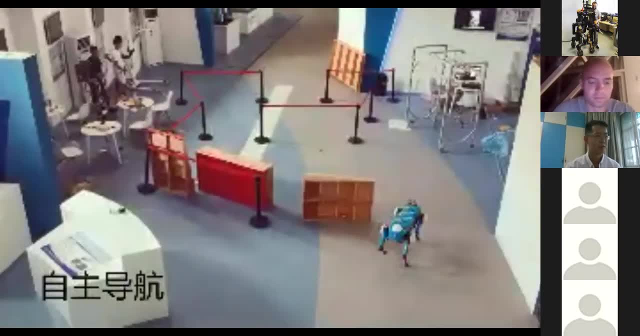 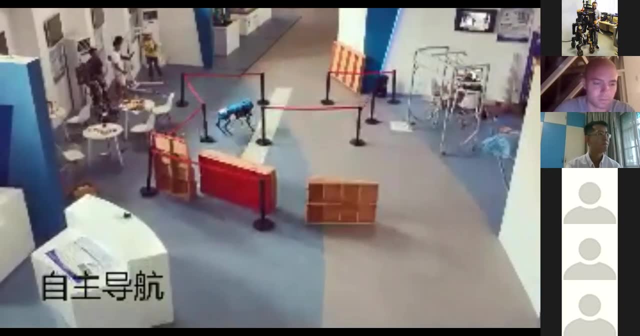 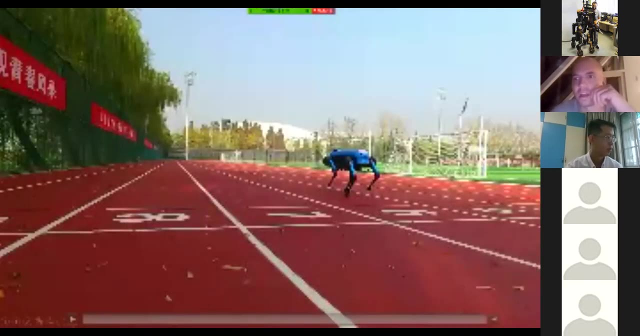 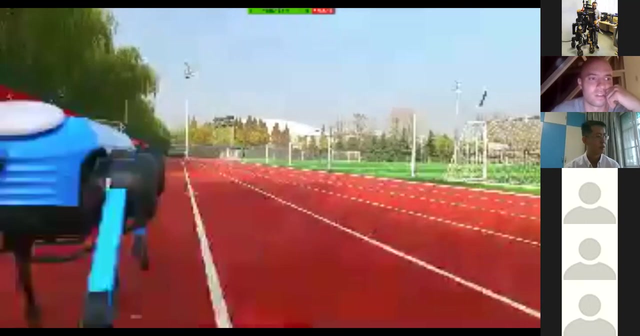 because you can't see it move. It's not like in the real time. Okay, let's see another video. is this the view? Okay, yes, we did that, it was good. more recent, it was in 2018.. As far as I know, it was the first robot in China- millions. 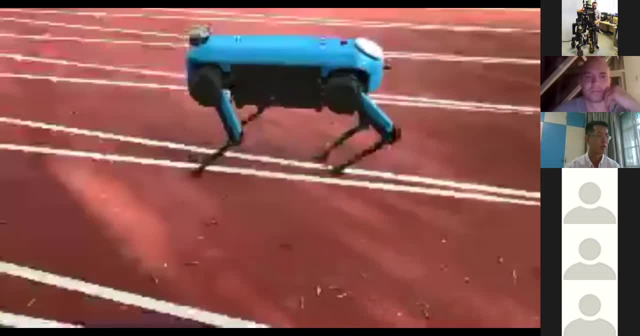 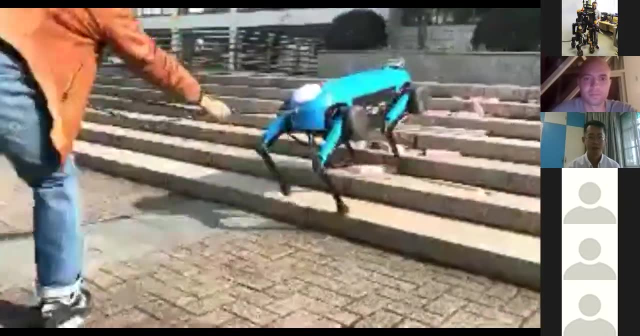 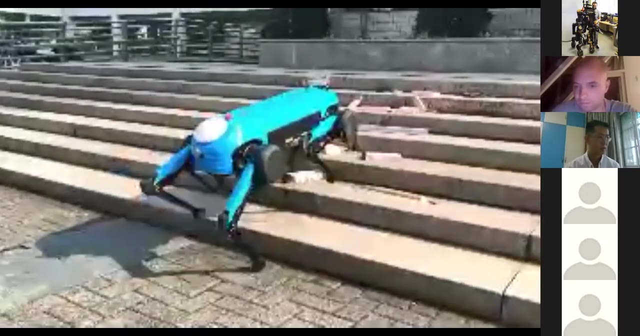 that can do this jump charting running with a full, flat face And also can get up the stairs. Also, the first robot in China, million, can do this And even though there are some small obstacles on the stairs, it can get up the stairs. 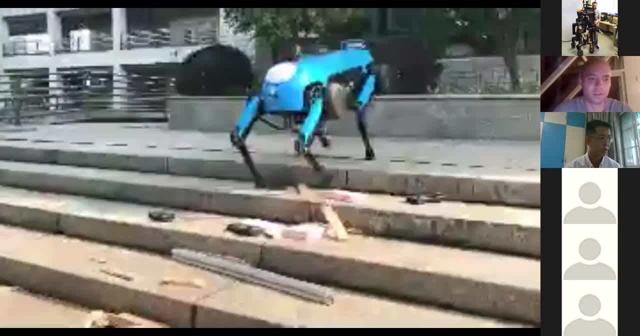 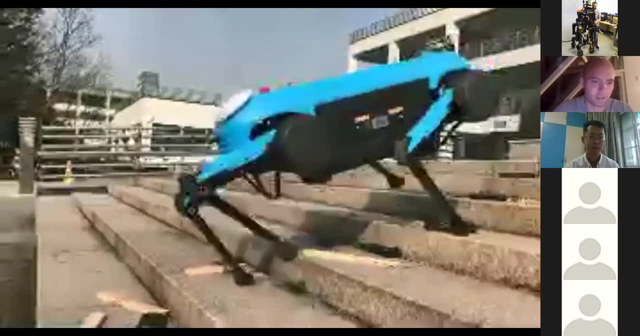 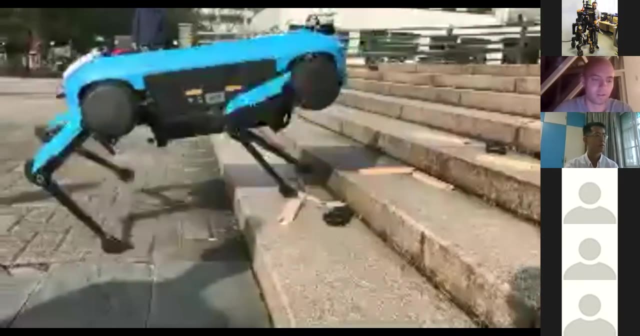 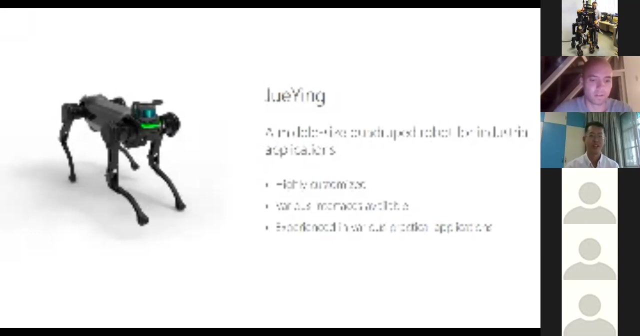 And the height of the stairs around like 10 centimeters. So clearly the so here we go with our standard product, Drane, and also the star product of ours is a middle-sized quadrupedal robot And we plan to use it. 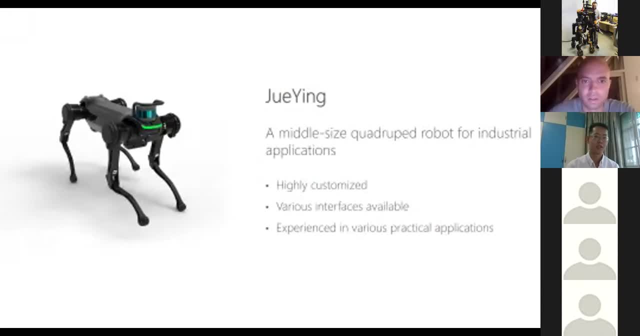 for some real industrial applications I'm going to introduce later in the followings. and it can be very highly customized. the customer can choose whatever he wants, want to add to this robot. as long as he can, he can afford it and he can. the robot can take to carry this weight and we can offer. 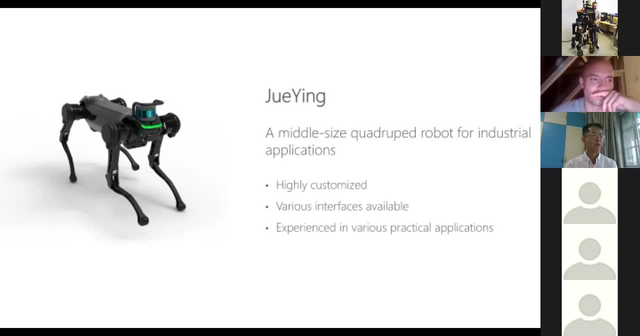 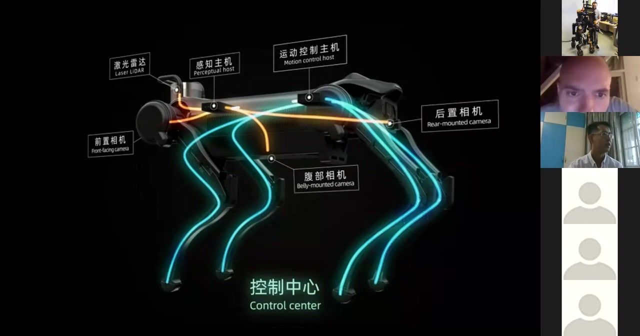 various interfaces and it's after this year's development. it connected a lot of experience in various practical applications. I'm gonna talk it in the following. first, let's see what we have as the default settings. we got a leader in the top top front and we got a three cameras in the front. 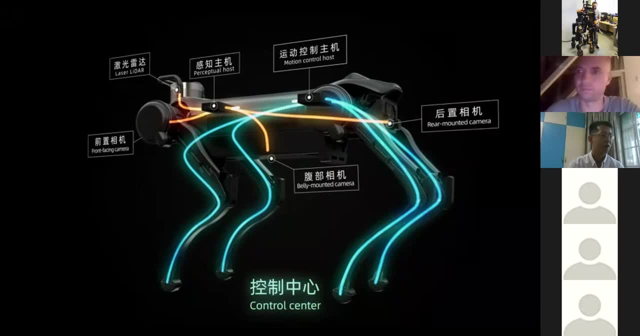 and we got a three cameras in the front and we got a three cameras in the front, in the back and also in the belly- what the belly camera is for I'm gonna talk about later with the video. and we saw also we got two hosts on board, one for. 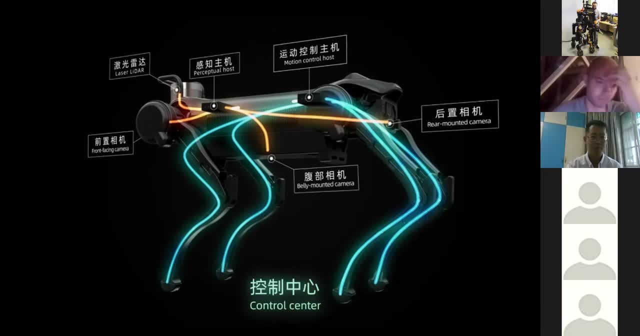 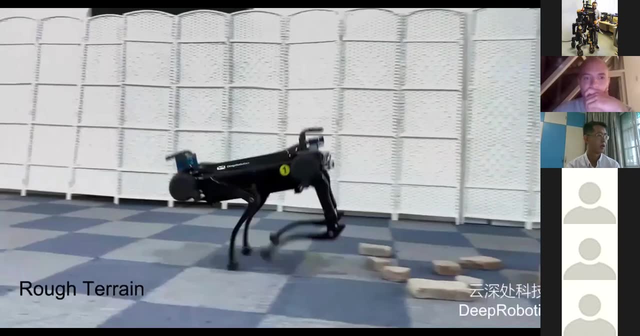 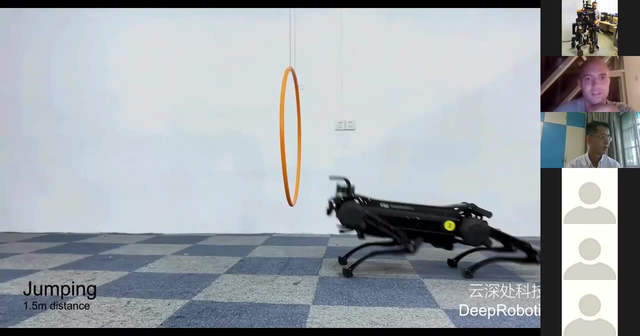 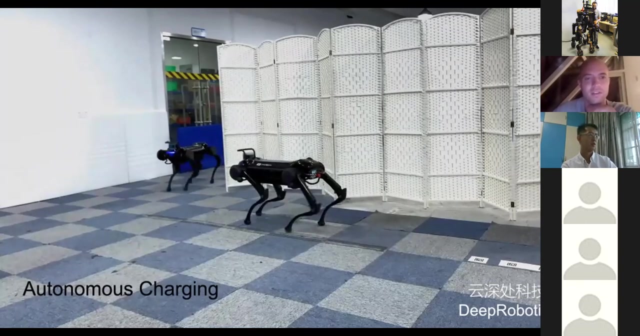 the perception and one for the motion control. let's see the video. see it's. it's funny through raftery and is so cold, so can jump very high and very long through a circle. through a circle it's a more than 1.5 meters in distance and it can also recognize another robot. 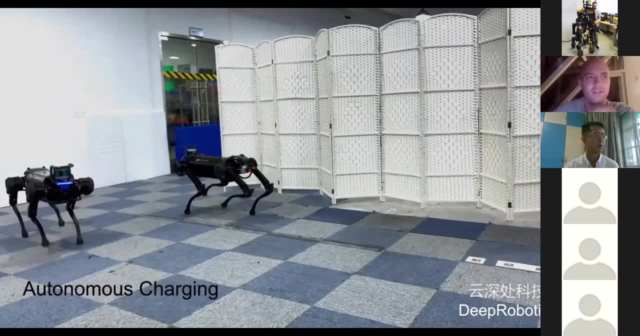 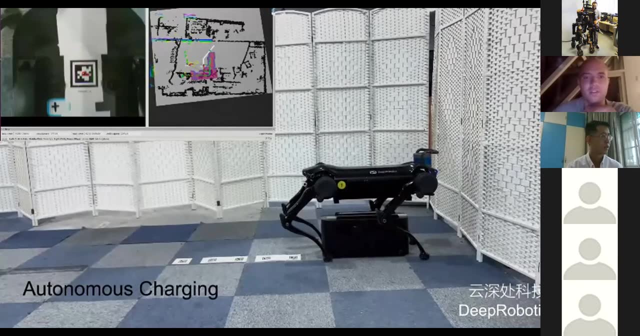 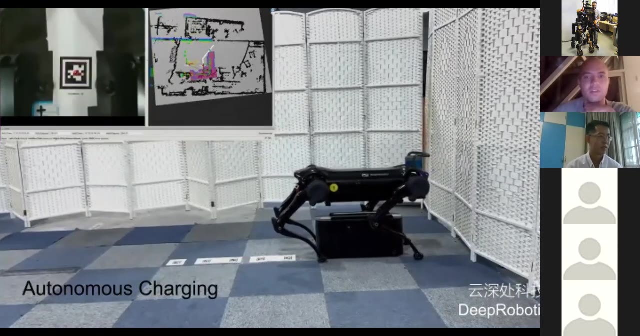 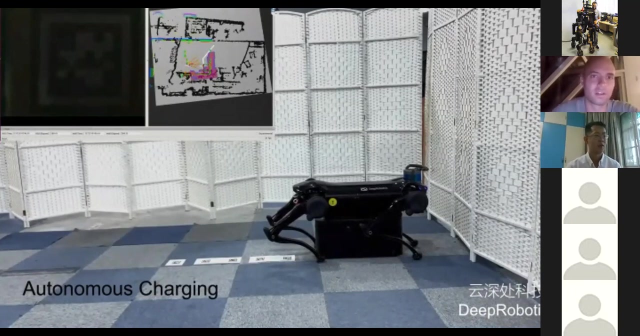 at the obstacles and the wider avoid the contact. then we plan a new path to his the station. see, see, there the belly camera is useful to get a better information about his position and the so that he can, so that each a length down and control his body position to. 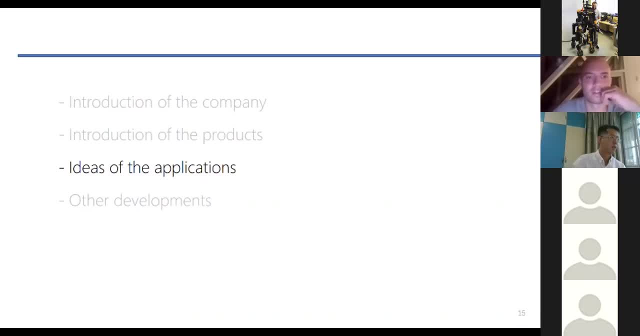 lend a accurate truth at plugin so that he can get charged and then looks to me. let me introduce our barriers of the applications. first problem is that: why do we do inspections to be the job out? the first problem is we can't catch that EP on the second last step. so first of all, briefly, another tip is that is to 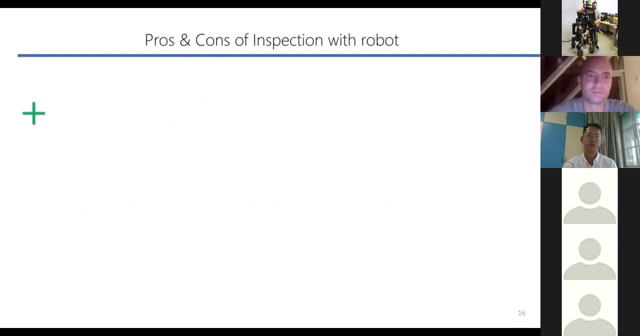 is the. it's a big market. if you google transformer substation in China- million- you will get this. it's more than thousands of it and in every of every one of this substation there are two or three personals that are in charge of the inspection, manually inspection and in the beginning of the product we hear: 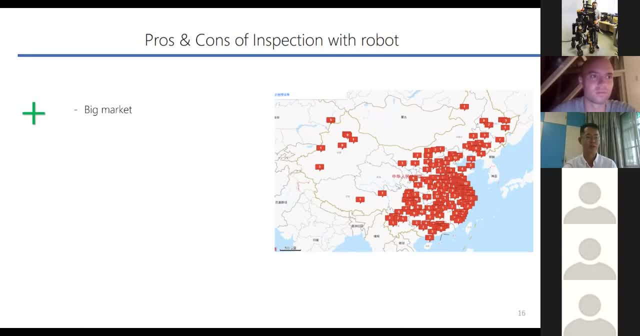 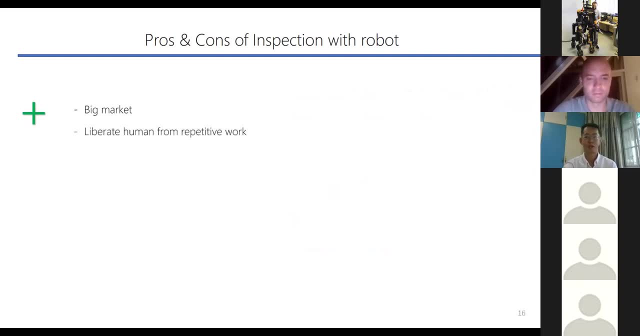 a lot of complaints about how the power in their work is. so inspection with robots. it can liberate human from the repetitive work, from the boring work, and after a few trainings the robot can give a relatively reliable diagonal diagnosis about the trouble and about the instrument or equipment. and it's also very costly effective compared with. 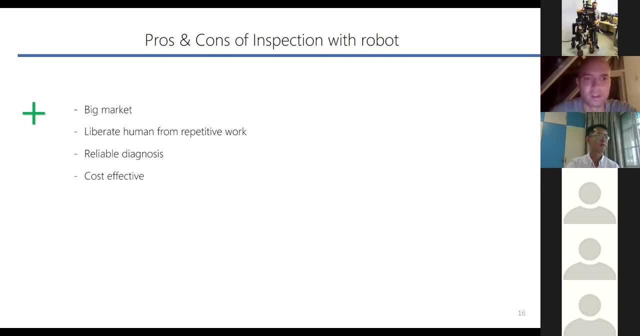 hiring a real human. but it also has some disadvantages, like great difficulty, great difficulty and the great difficulty. so all the troubles caused with the difficulties, because when a robot step out of the lab, it's the things are getting different, the environment is not so ideal and not so. 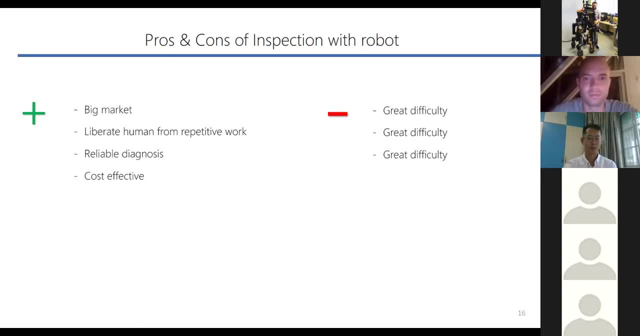 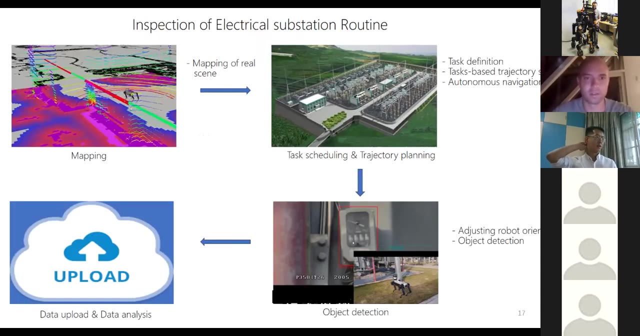 good as in the lab. so we faced a lot of this very practical and project problems, but we have fixed them and we are processing- and this is a routine of an inspection of electrical substation. we have to build a map of the real thing, use the radar information and then 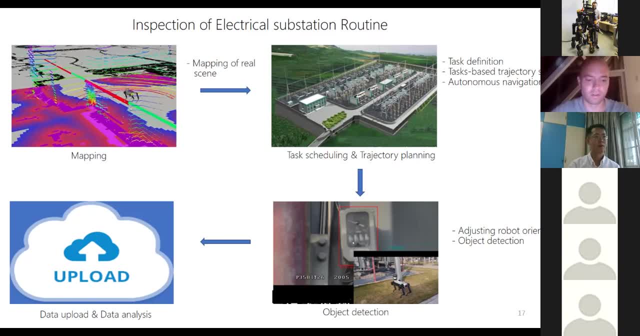 we're gonna define some tasks, whether the robot is going to do a routine inspection, daily routine inspection, or it's gonna do a specific inspection to to go to the specific place to check the state of equipment or or a instrument, and after the task definition, the robot can build a plan, a plan path to go to the 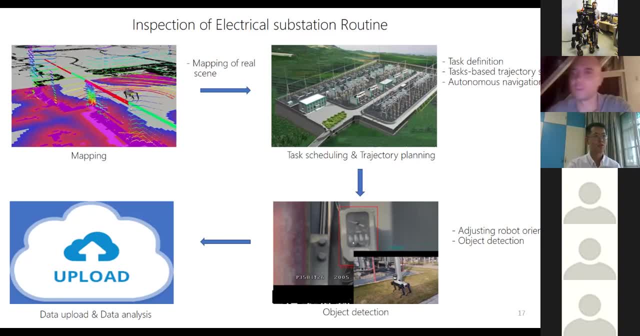 right place and then the robot do the autonomous navigation when he moving and when the robot goes to the right place and he will adjust his body position to let the cameras or the meters, terameters- to have a good direction to the object and then to the object detection and take pictures and information or data of 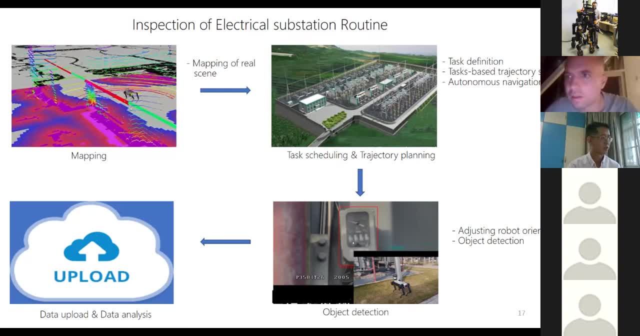 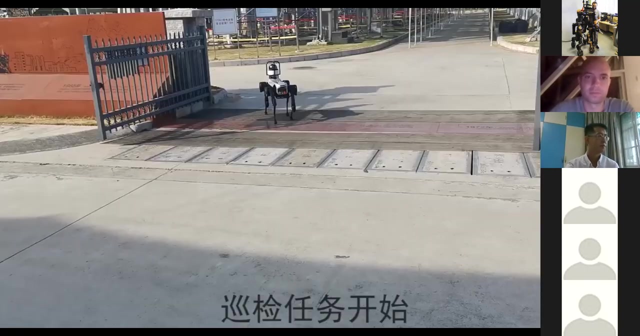 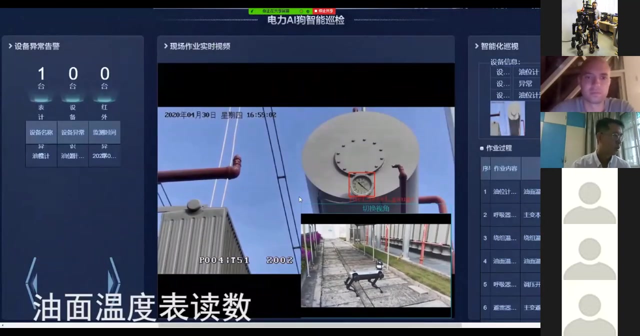 the instrument and then to upload all the data and information to the, to the cloud, and we will do some data data analysis with this data. so let's see the videos of the real applications. the mission started and then here he came, to a all your level meter and take the. 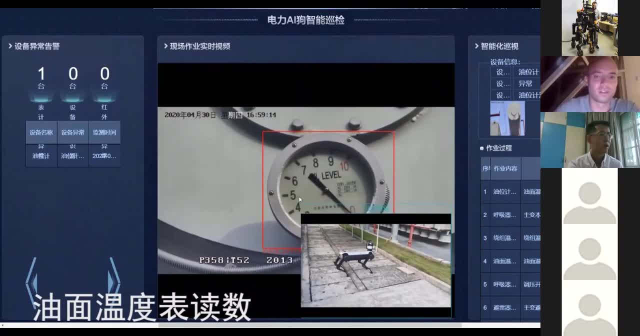 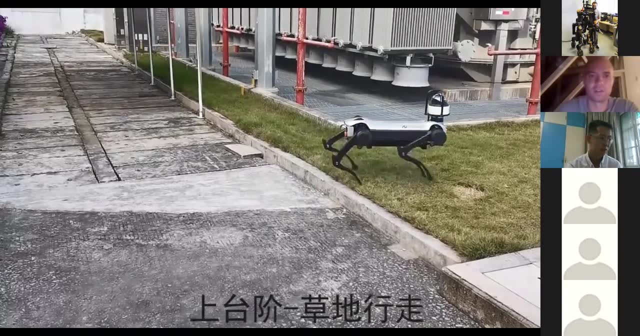 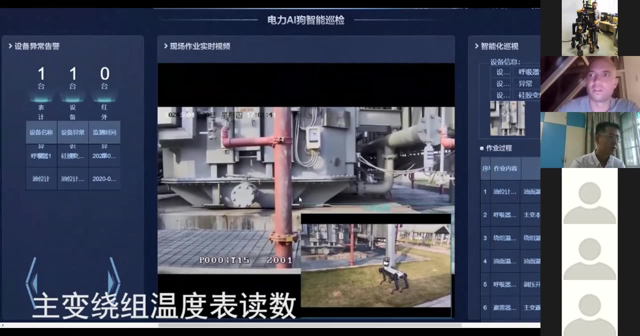 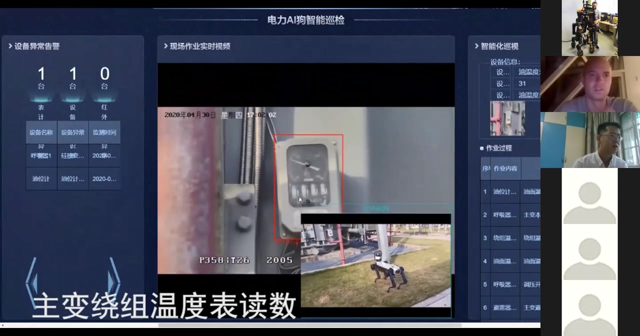 pictures. and then he left. and he came to a all your level meter and take the pictures. and then he left and and getting on a road shoulder and walking through grassland to another place to take some photos and data with these mirrors. It's a thermometer. 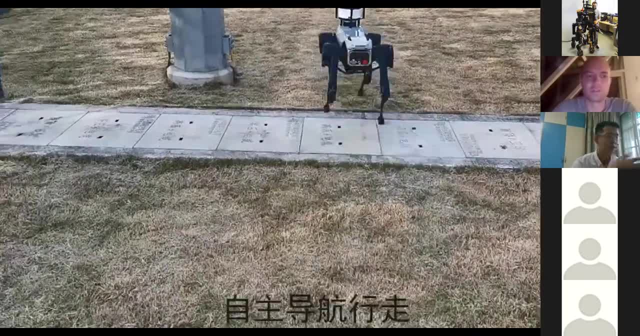 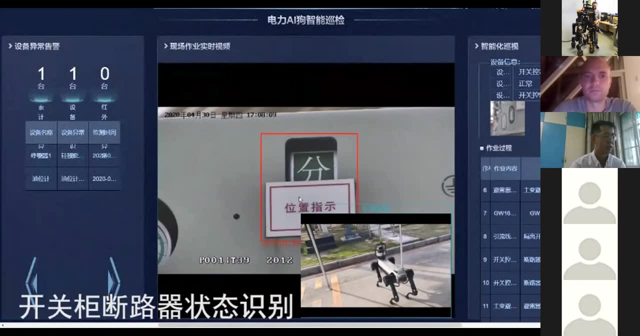 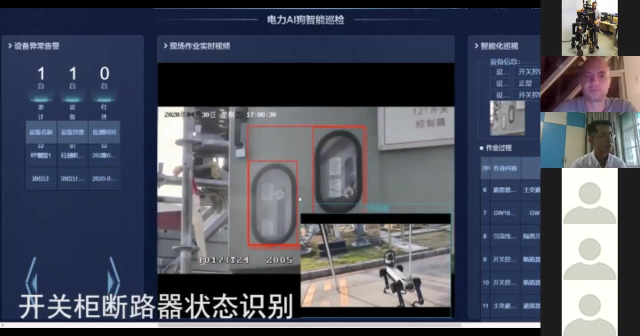 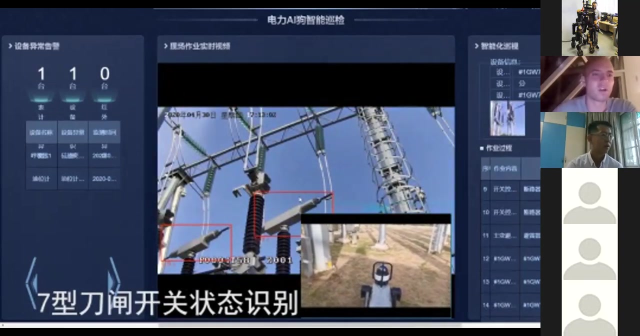 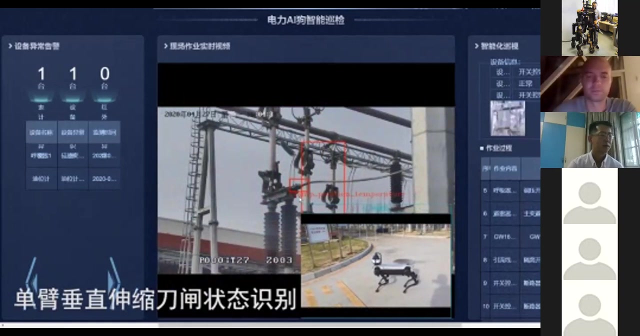 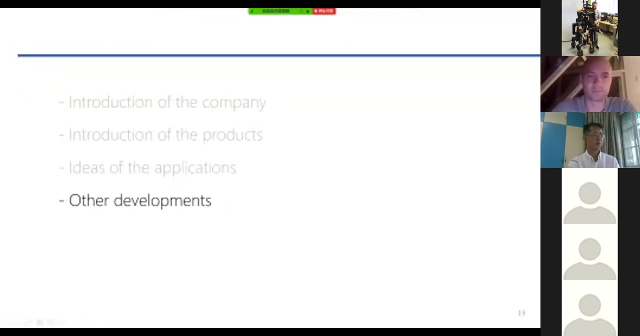 and you can do the autonomous navigation in this place and to check whether the switch are in the right places, and also this kind of equipped equipment. Okay, the applications was introduced, finished And some other developments also has been developed like this: the localization under very strong shakes. 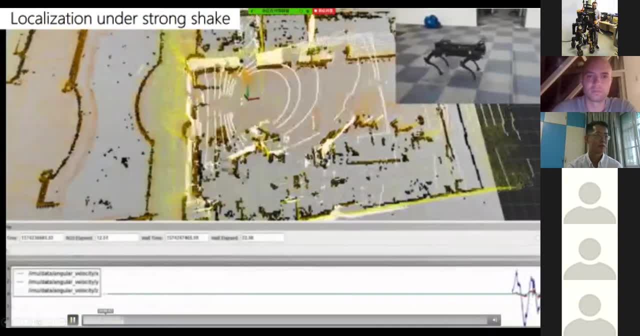 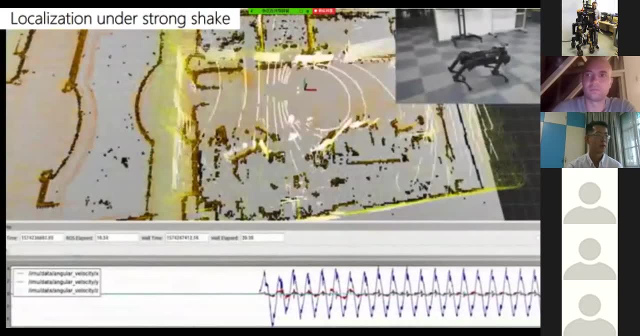 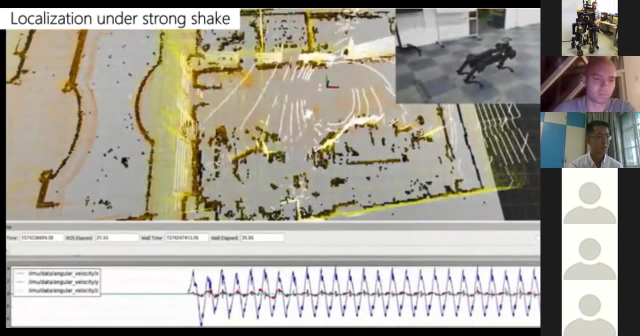 Let's see it first. Yeah, we can see, because we know the robot. when he's moving or doing some particular projects, the body can move very, under a very strong shake. But when you're in this, when the robot is in this kind of state, 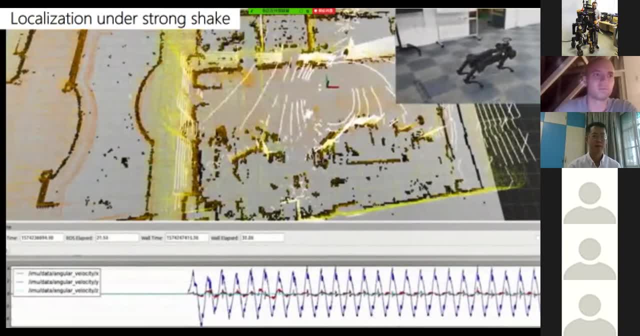 how the robot can navigate and localize his positions in the environment. it's a tough task Because we have met a problem with when the robot want to get up a road shoulder after a slippery. the robot cannot fall, but gonna slide away with a very quick speed. 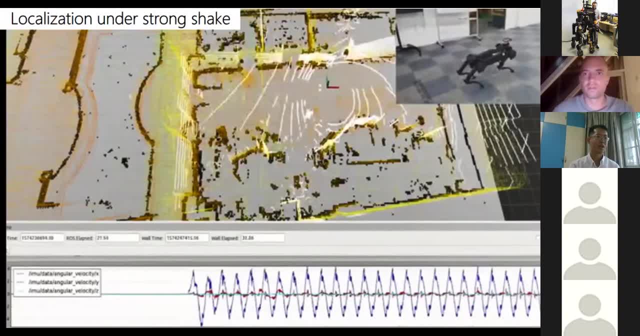 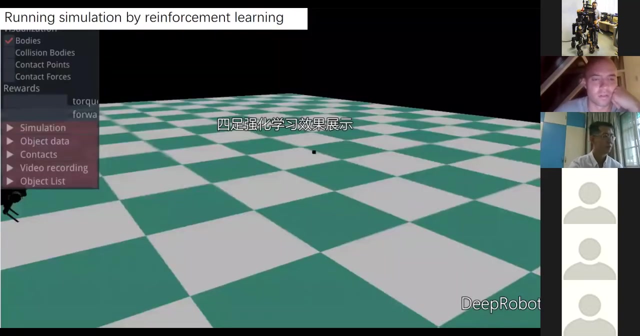 And in that time, sometimes the robot can lose his navigation, lose his localization, And once we do this, after we have done this, the robot can still localization itself in when he got asleep- Okay, Sleepy, And this is a running simulation. 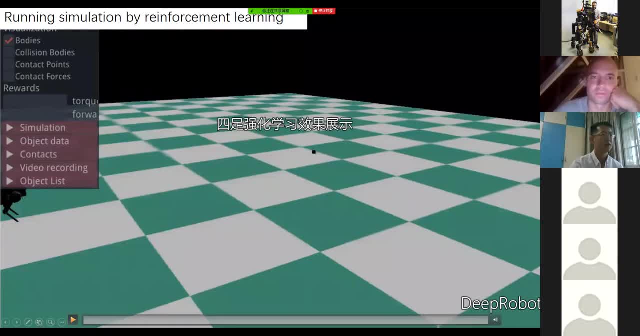 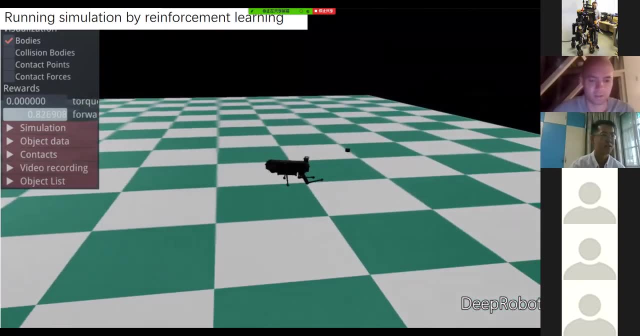 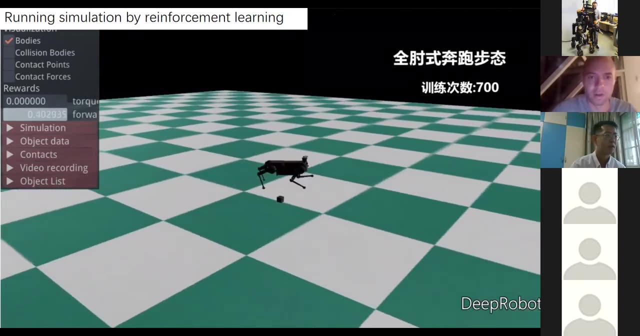 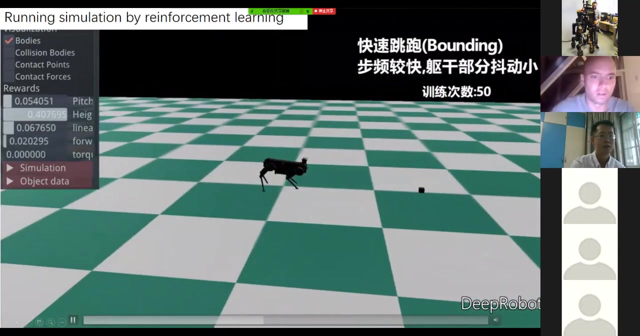 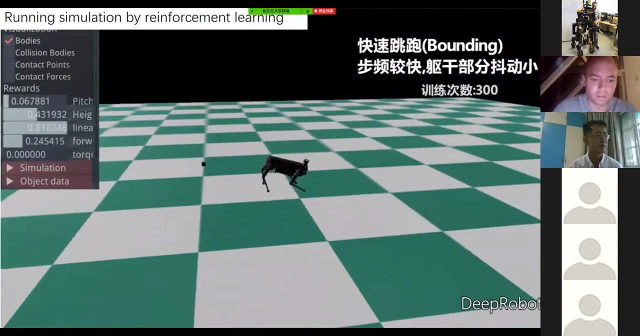 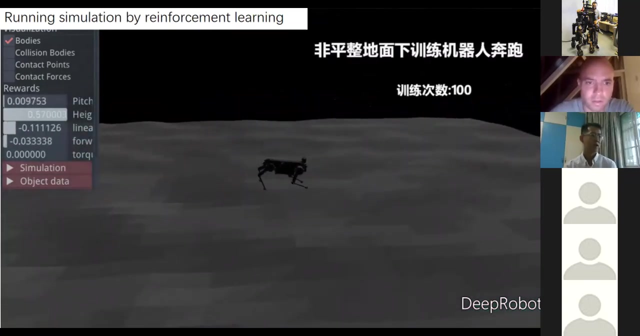 by the reinforcement learning. After 500,, 2,000 to 12 training cycles, the robot can run like this And this the running gates. like our robot, It's trained for the bounding. Yeah, after that, we have trained it for the. 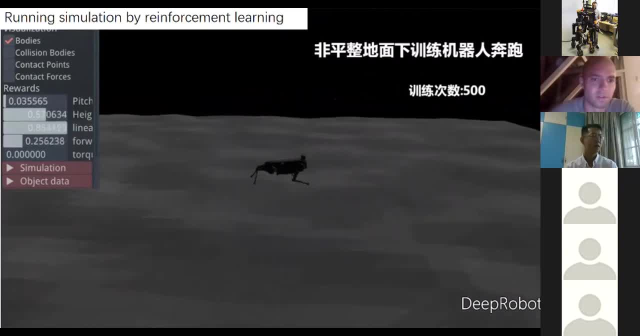 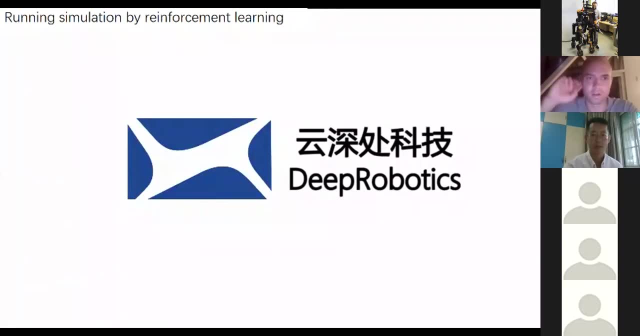 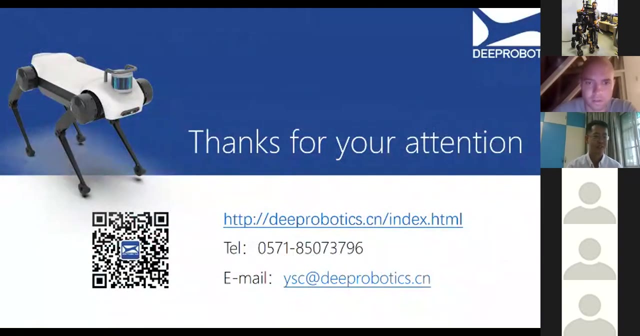 in the regular terrace. After a few trainings, the robot can run very quickly and very stable. And that's it. My talk is finished and thanks for your attention and time, And if you have further questions, I'm glad to answer it. 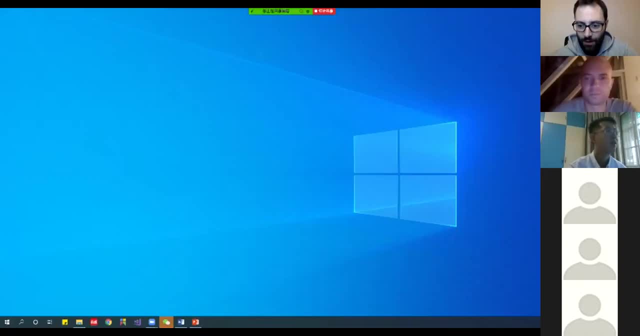 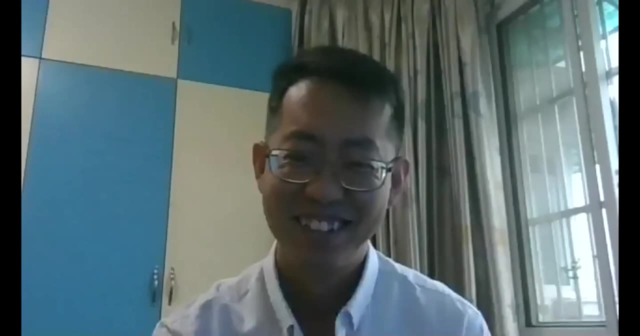 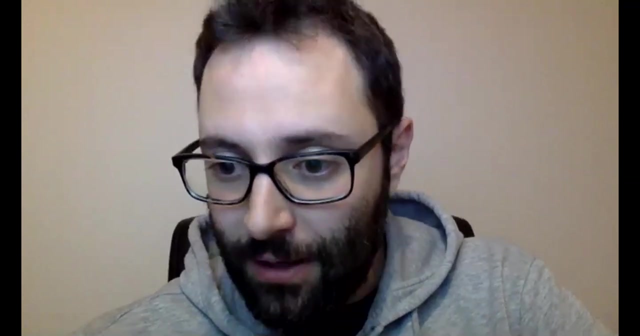 Thank you. Thank you very much, Jingyu. Thank you too. This was a really really nice talk. Thank you, Very cool things. Okay, everybody. if you have questions, please feel free to start asking them in the chat. 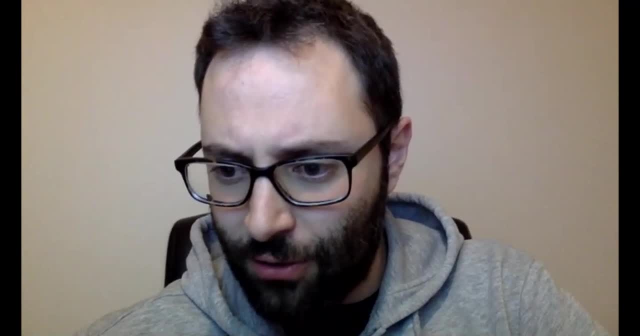 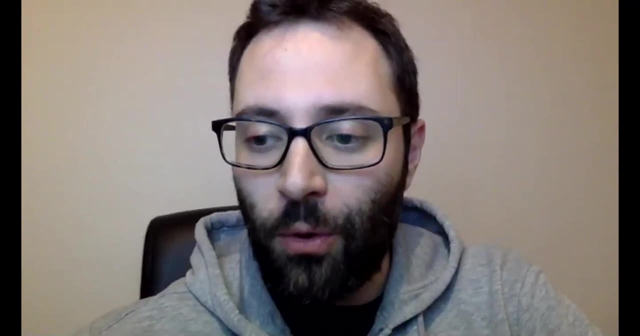 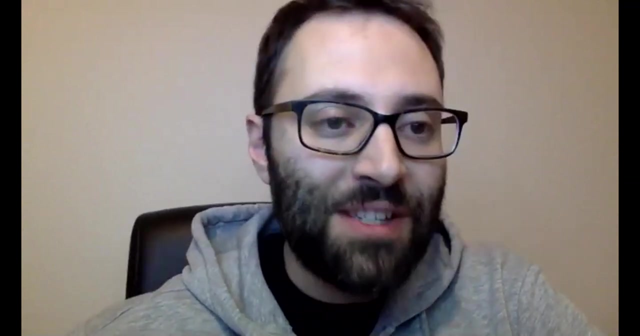 We got some questions from our site, so let me go one by one. Okay, the first question is actually about the bipedal robot, the Wukong. So Marco is wondering that we have not seen too much information and too many videos regarding this robot. 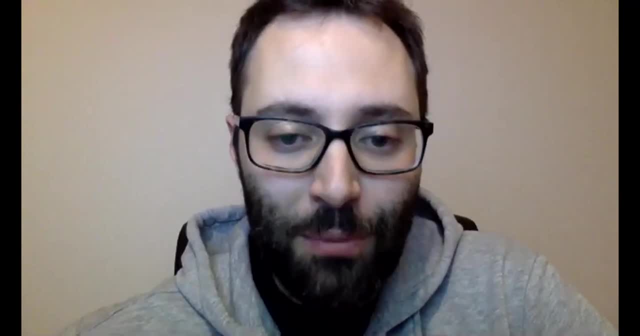 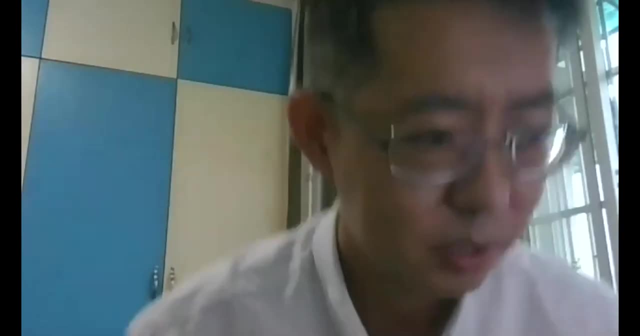 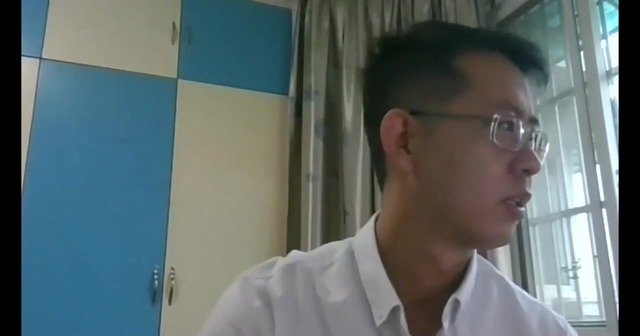 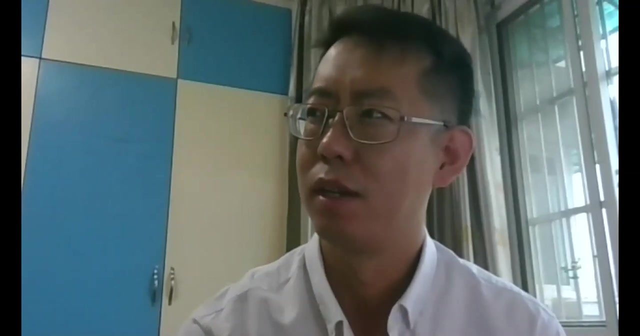 I mean, can we find some informations about the information about the, the humanoid robot, the Wukong? yeah, of course, but actually it was developed in before 2012, I'm wonder. I'm wondering that maybe there's not so much videos and pictures on the internet, but I'm sure that Dr Zhuqiu Guo has some of. 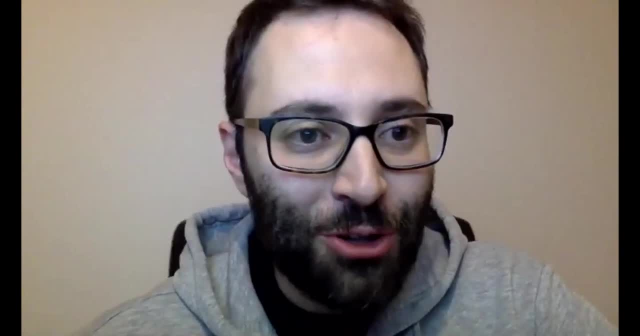 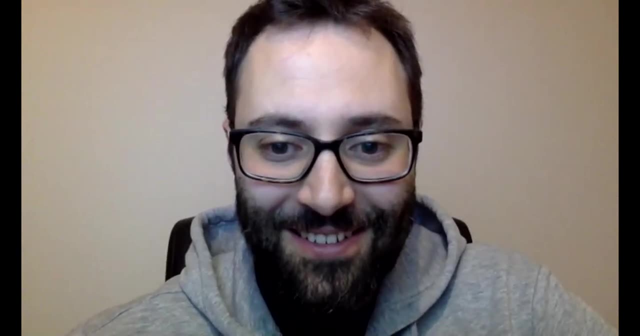 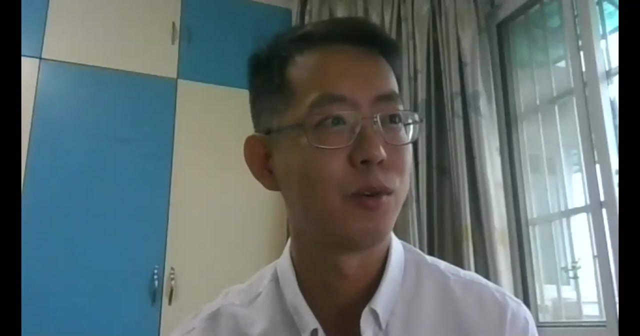 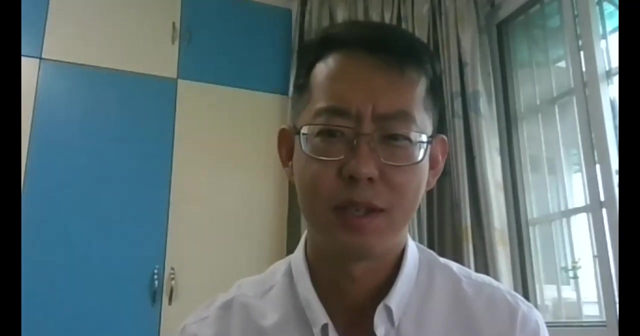 this all right. you showed also a newer version. no, I thought it was a 2018 version. no, in your slide you mean the second generation, right? yes, the second generation. yes, they are developing it right now with the progress. let me see, maybe maybe on his on the homepage of the university, maybe you can. 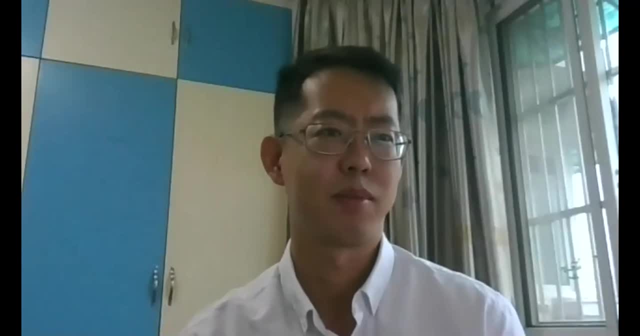 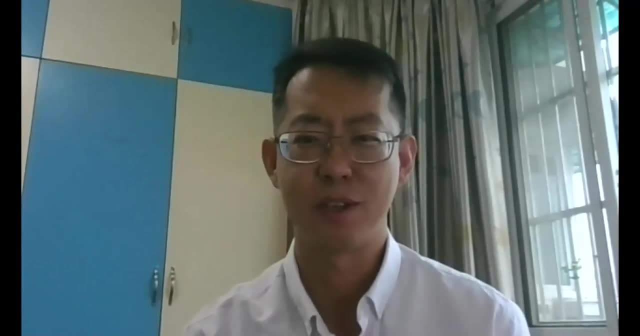 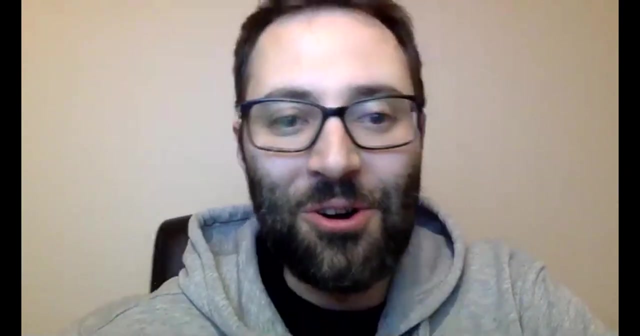 find some, but it's all in the media's place. it's hard to. it's hard to organize this information together, you know. but if you are really, really interested, we can. I can ask Dr Zhuqiu Guo to offer some. no, it's very interesting because it's very 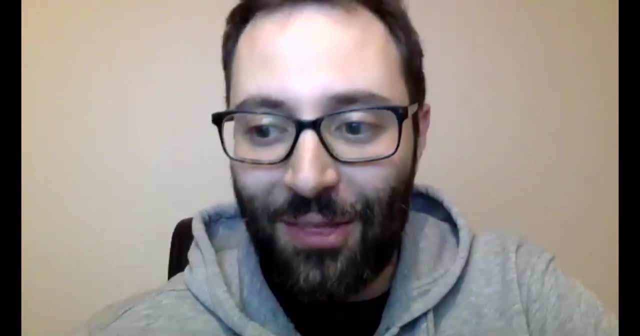 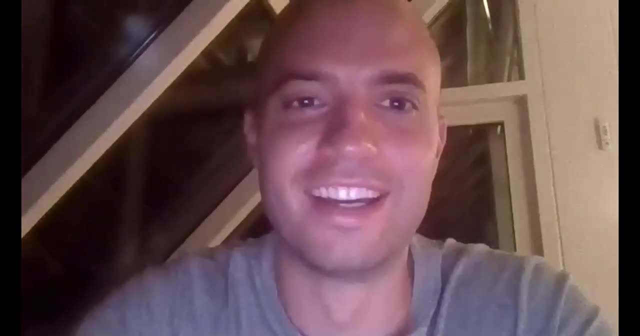 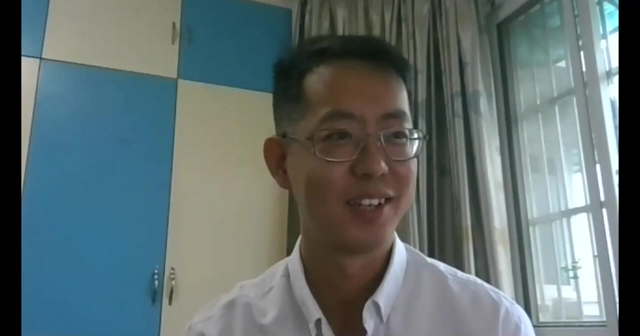 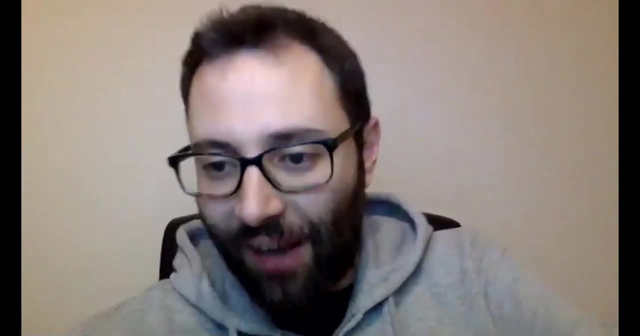 interesting because I don't know. also, Marco, I didn't have any idea that this humanoid exists actually, so, especially from the pictures, it looks looks like a great product already. thank you, thank you, yeah, but it was basically mainly developed in the University and right now we are a company, so we basically developed the quadrupedal robot. all right, okay, okay, so another. 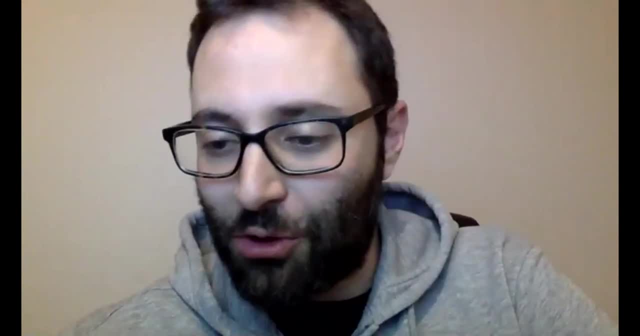 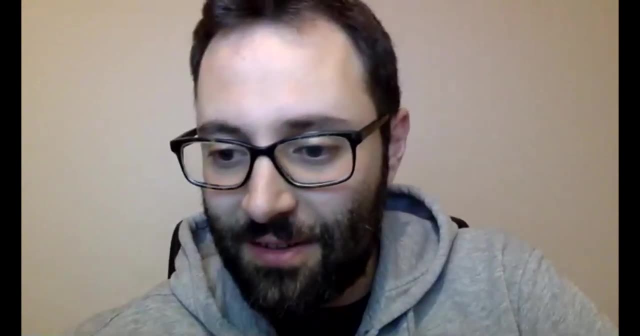 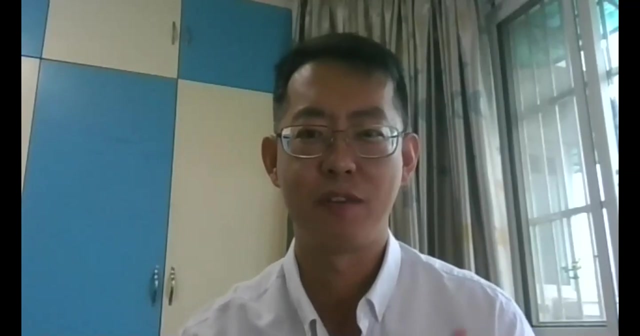 question from Marco is- and if you can talk about this, I'm not sure- what is the price of the quadrupedal robots? what is the scale of the price? it depends, because the all depends, the small one, the large one, and depends on what kind of options you want to choose. but let me see, it's around you. 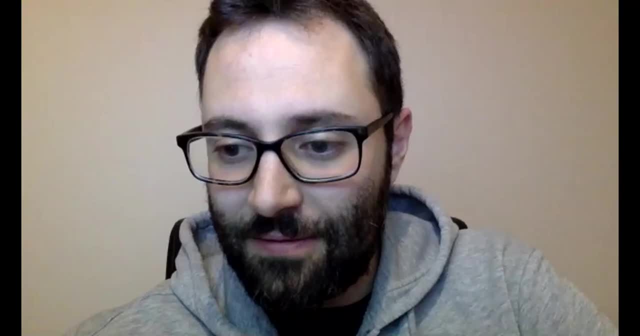 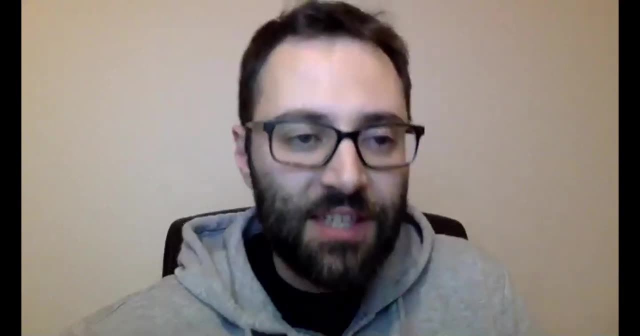 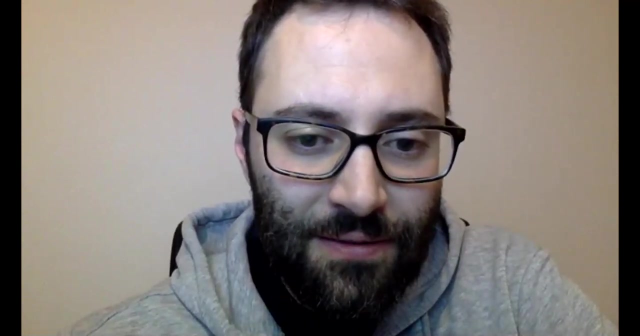 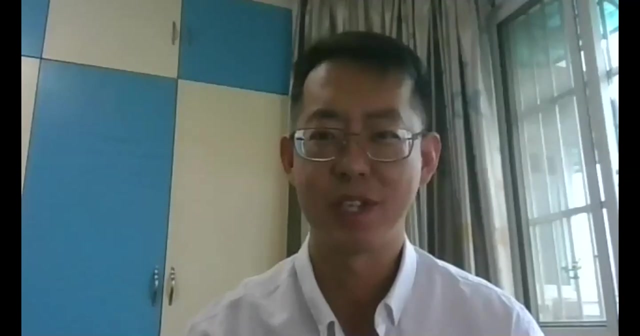 use dollars right. yes, let's say yes. approximation, I mean, is it closer to 50k, 100k, 200k? it's around $5,000, maybe cheaper, I'm not sure, because I'm not doing the market part, okay. okay, are you selling? are you selling worldwide now, or only in China? 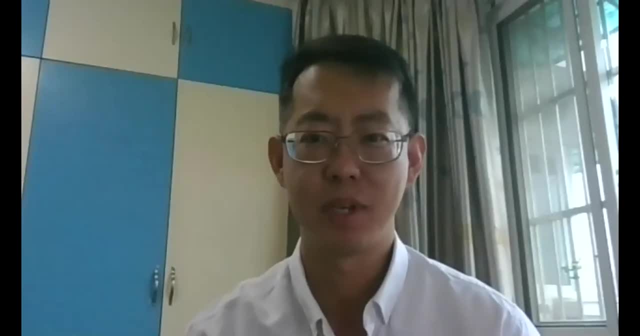 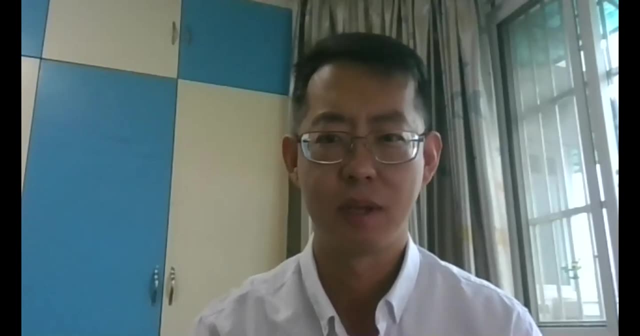 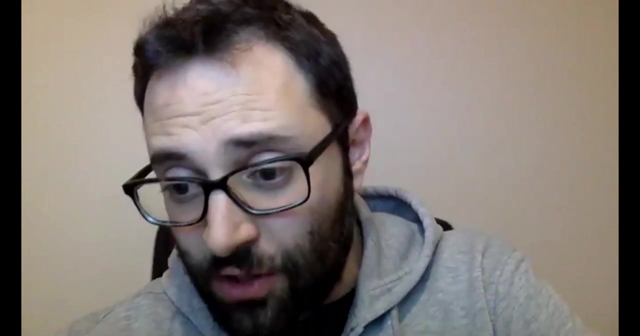 yeah, not only in China. we have some partners in Europe, but I'm not sure that we have partners with USA. but we are planning to sell it worldwide. all right, perfect, all right, let me see. I mean, one question from my side was that, of course, maybe you, you, it is something that you 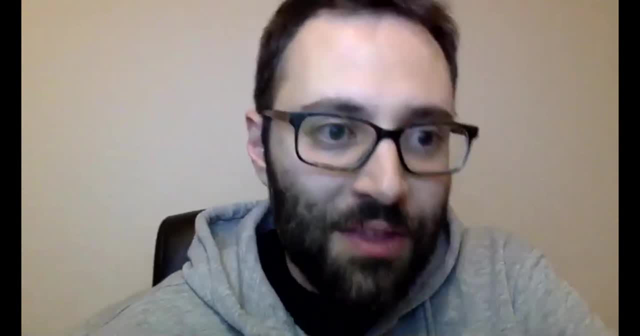 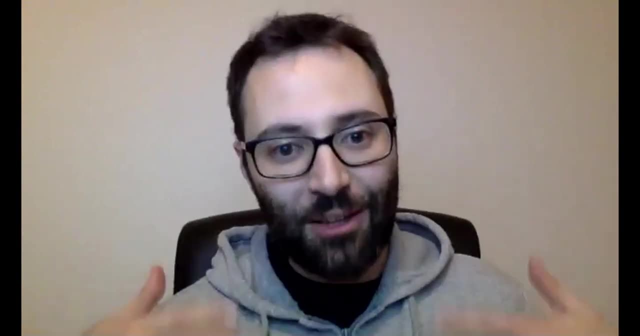 developed now the arm on the robot. so this is, this is a nice, interesting idea that I know a lot of people in you know in quadrupedal robots are trying to develop. I mean we have seen also from Boston Dynamics animal also HiQ, etcck. is this a challenging thing? I mean putting a- including nella, which I've talked of in other videos have been fast reused- or also enjoy giving money to the population and so forth. well, I will test it and see which to do is the best to choose. okay, so I hope to absolutely not take it Isey. you say yes if we are the worst to say agree at all. so have one question right now. so please talk about the overall pot of the специ cheat for 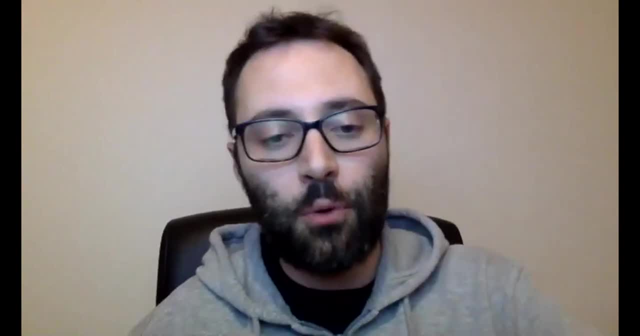 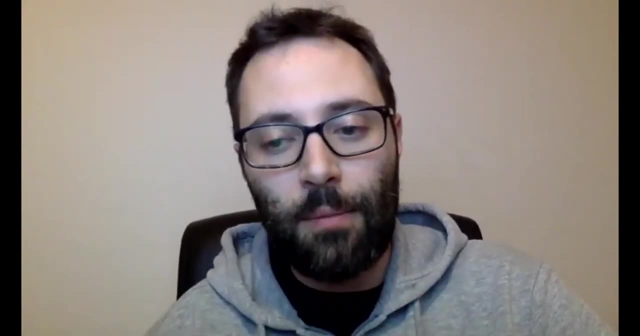 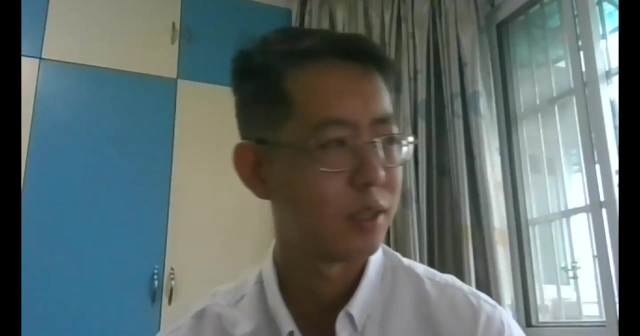 Is this a challenging thing? I mean including the dynamics of the arm in the controller. does this make the whole control much more difficult? you think, Yeah, yeah, of course it makes the controller much difficult, And you know when the robot 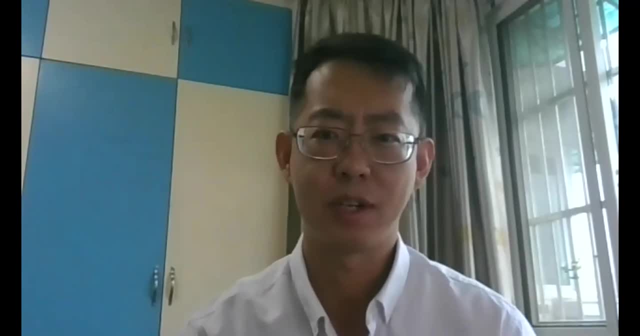 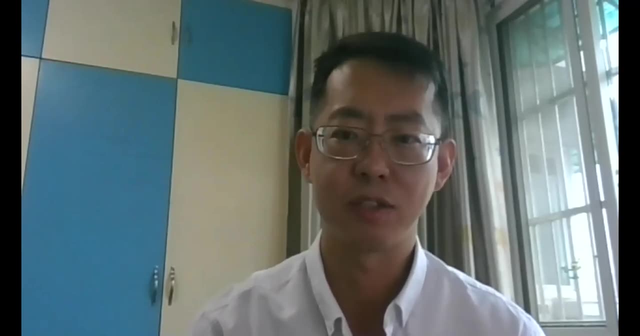 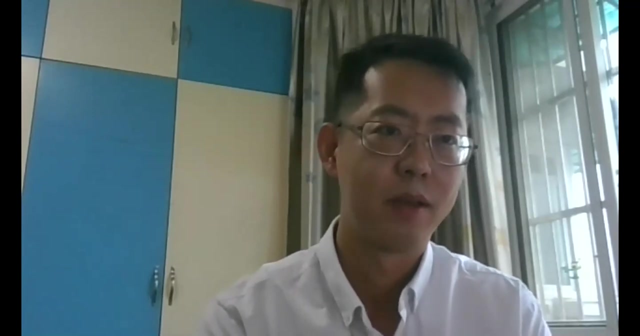 has the arm. the arm has various configurations And under every configuration the robot must to balance himself as usual. That means that you have to the robot must know how the configuration of the robot of the arm and balance itself accordingly. And even though it became much, 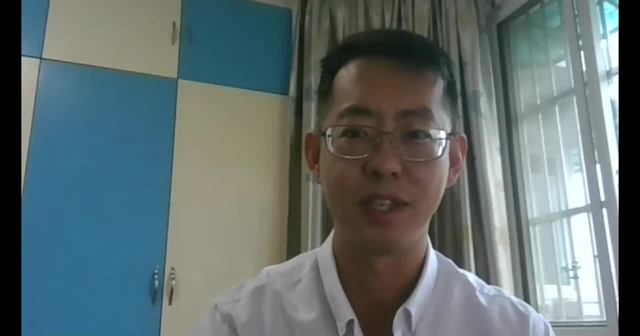 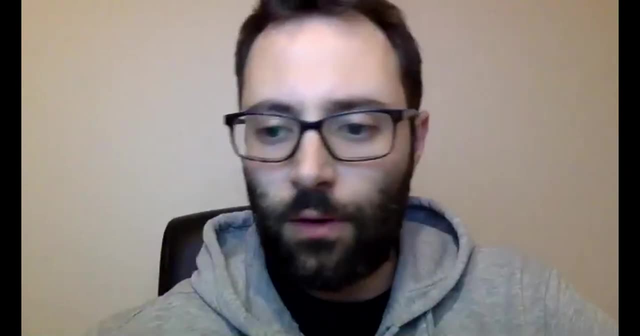 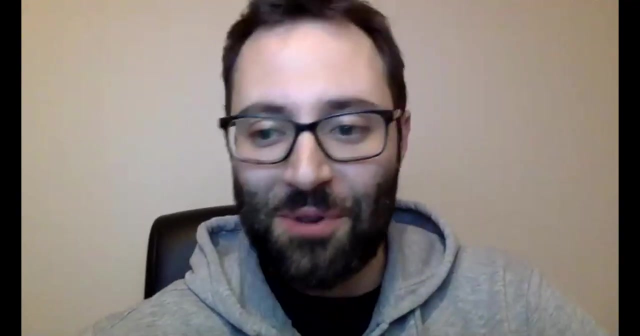 more difficult. when the robot arm gets something in his hand, you know it changes the initial momentum totally. So we are under development. All right, great, Okay. I mean we look forward for this. It looked nice in the videos. 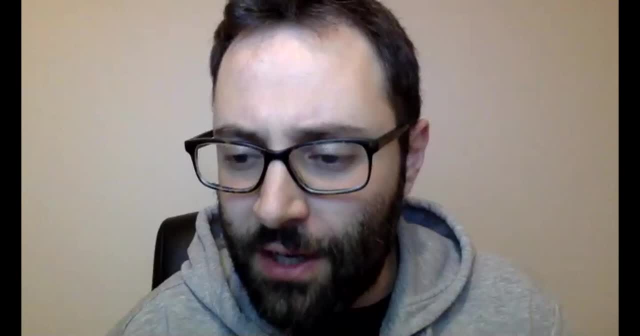 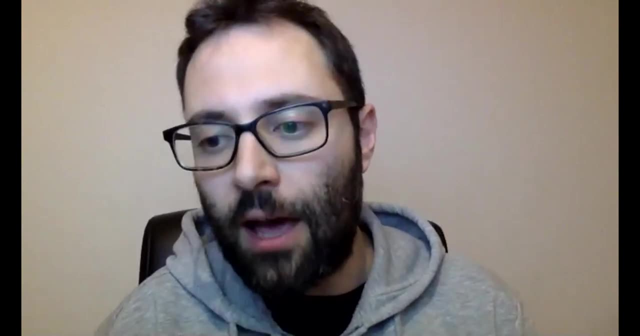 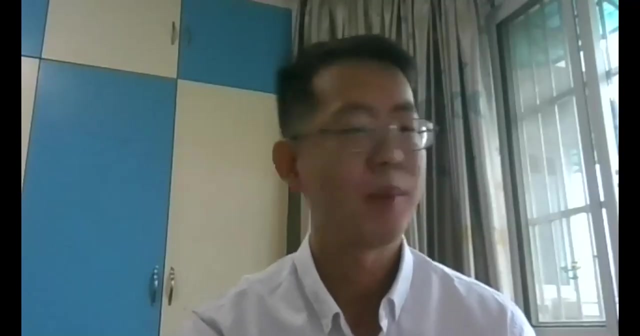 Thank you. thank you very much. One question, also from Marco, is if you can tell us a little bit more about the locomotion controller. Is it based on optimization methods, MPC, any learning-based controller? Okay, it's various, For example, for wheel, I think the MPC controller that is very good for the very high dynamic. 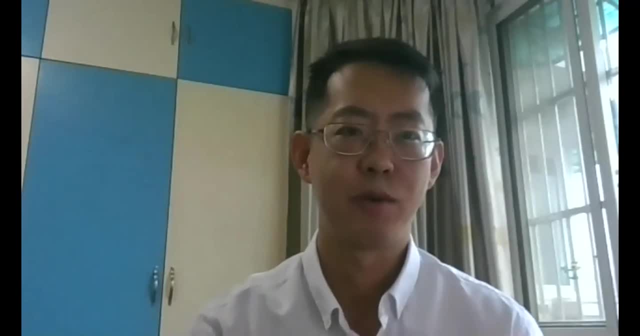 motions, When you want to do very fast runnings or when you're gonna step a stone or something like this. it can keep balance And the MPC controller is very good. And when we do the bonding- as you can see in the video, when the robot do the bonding- we use MPC controller. 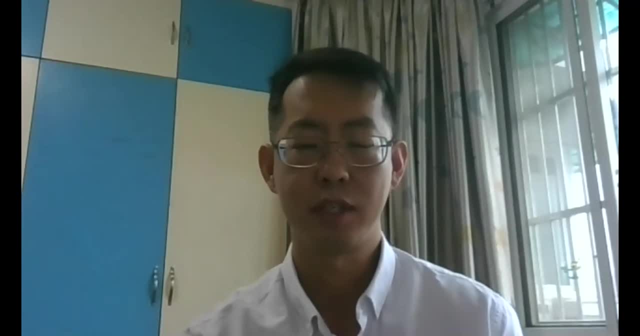 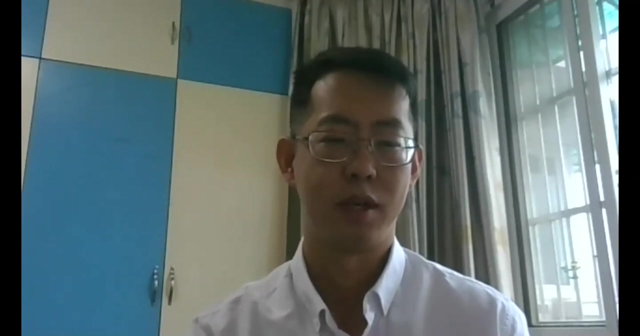 Okay Okay, But in other places we use our original traditional controller, like the virtual force, you know, just a virtual model of the robot- and to keep it balanced, And we think it's very good to differ the methods from the missions that you want to achieve. 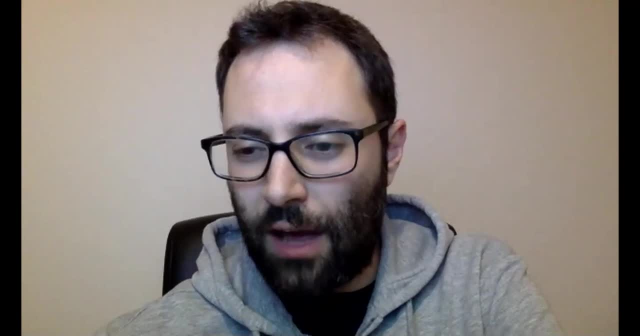 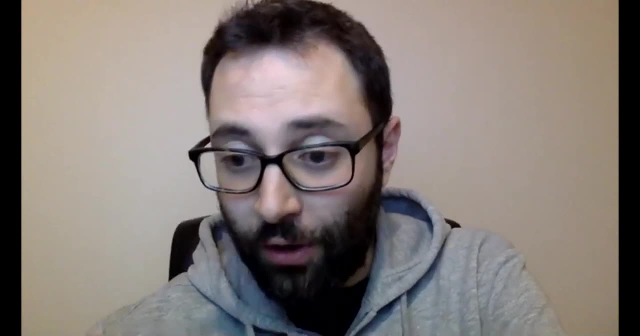 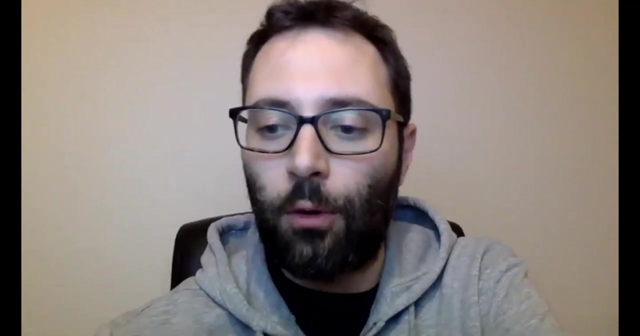 All right, okay, Great, I think. the other one, the questions about the path planning. I think you answered this, I mean, I've seen it later, Okay, so another question is: what do you think is the advantage of your selling point compared to other quadrupedal robot companies? I mean, 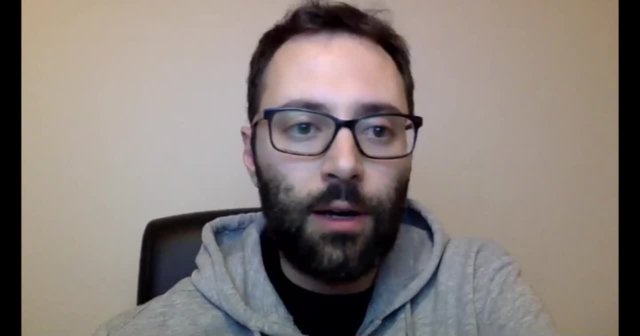 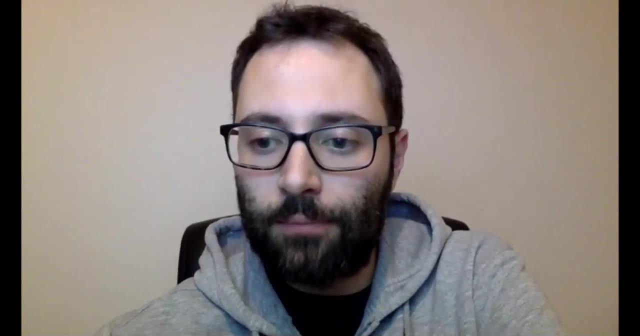 what is the advantage of this particular you know robot and the capabilities compared to other, probably compared to other, to other robots, Okay, Okay, so the advantage of this particular you know robot and the capabilities compared to other robots. 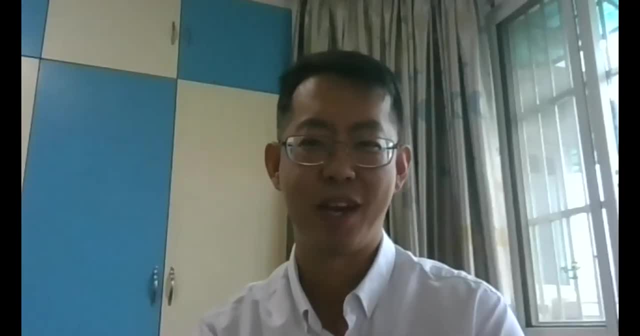 Okay, so the advantage of this particular you know robot and the capabilities compared to other robots. Okay, yeah, Recently there's many, many more companies doing the quadrupedal robot And we are glad to see that and we want to promote this process of the development. 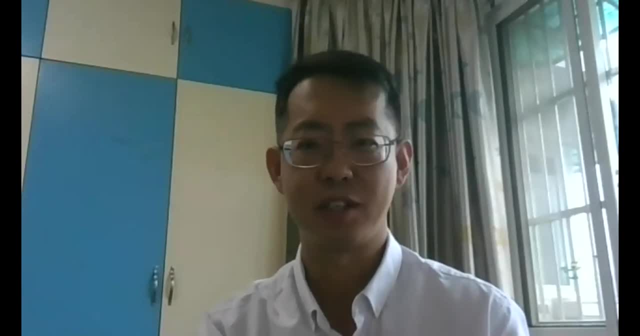 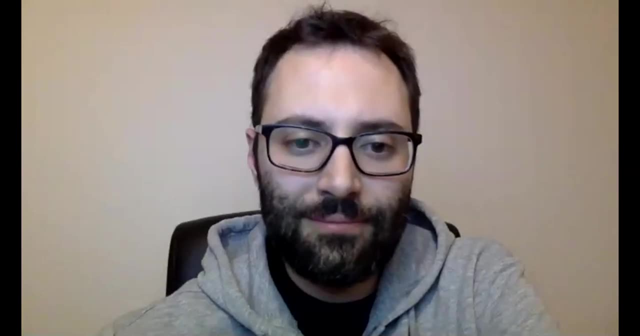 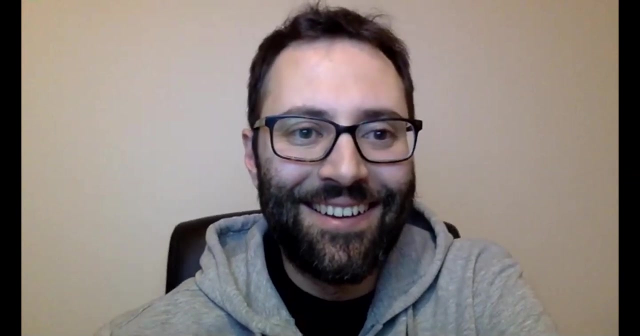 of the quadrupedal robot and we can all take advantage from this progress, right, And if you're talking about the differences, I don't. I don't see much differences about the, you know, the quadrupedal, It all has four legs and also can do the things And what we want. 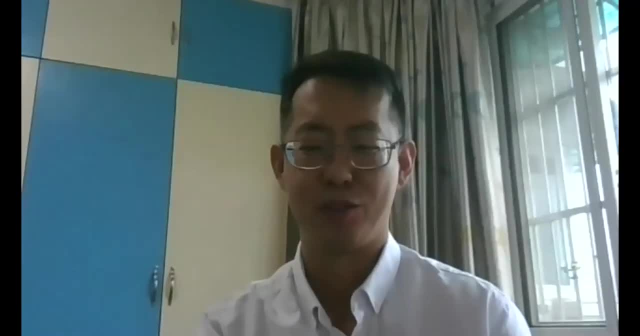 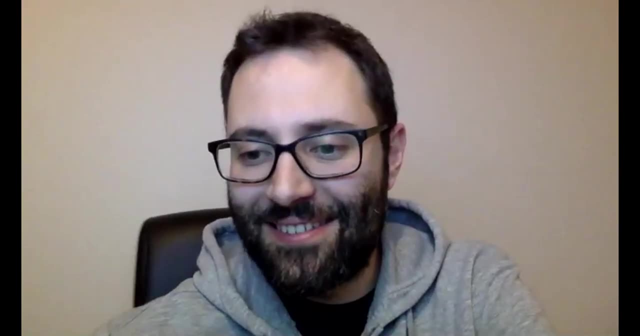 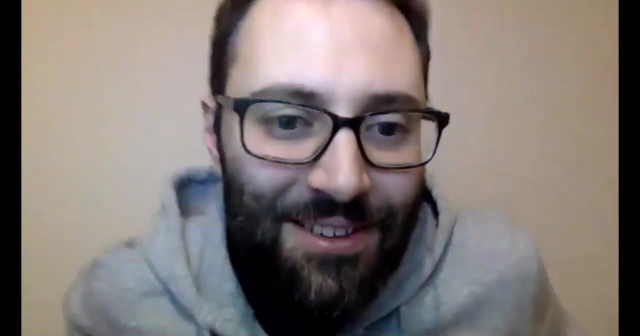 to do and they want to do it too. You know what I mean. Yeah, we want to do the applications and they want to do the applications too. And I think it's a good atmosphere. We can compare with each other and compact with each other, you know. 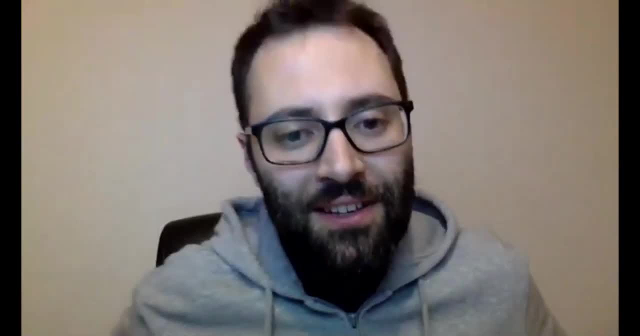 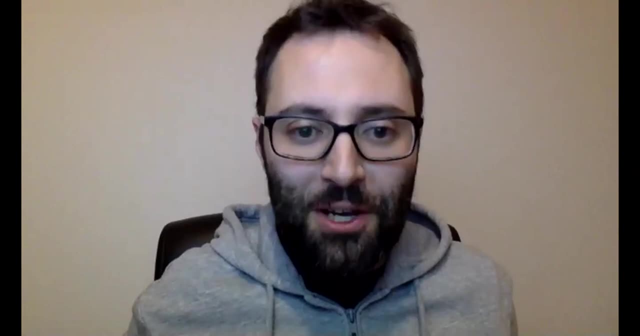 All right, that's fair. That's fair. How big is the company? How many people? How many people? How many people It's? it's around a 30%. Oh, you're quite a big company actually. Yeah, we grow, we grow. 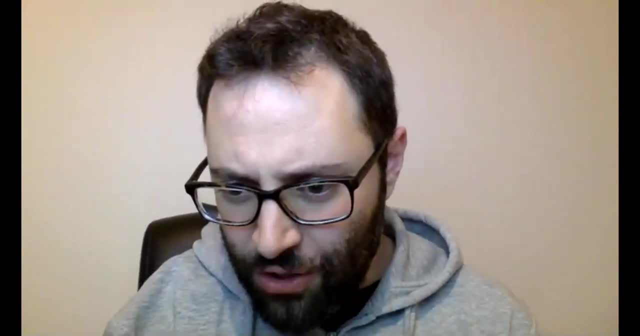 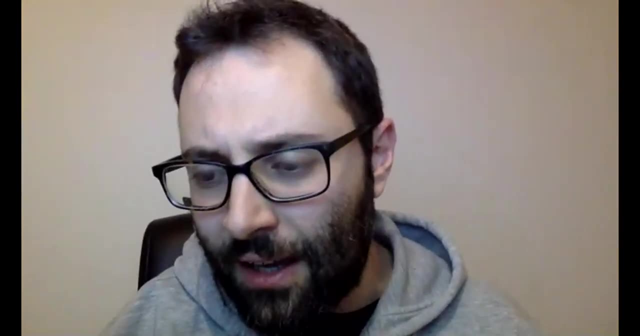 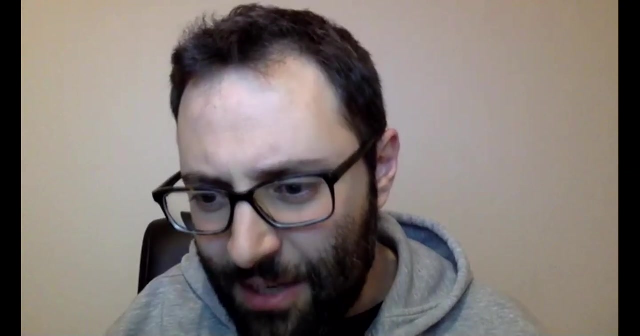 All right, That's. that's nice. One question from Mingxuan: Can you talk about the interesting tibia design? the curve compared to other, quadrupeds straight. It seems like it could be useful with the touchdown angle, but it's pretty hard. 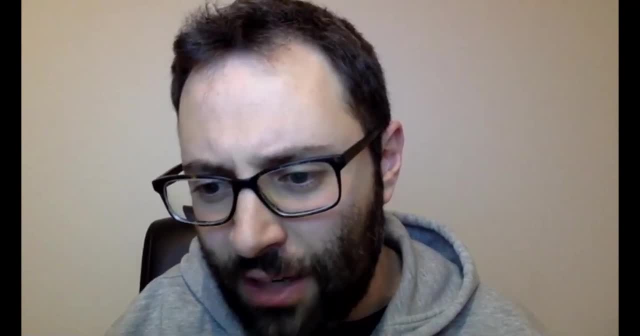 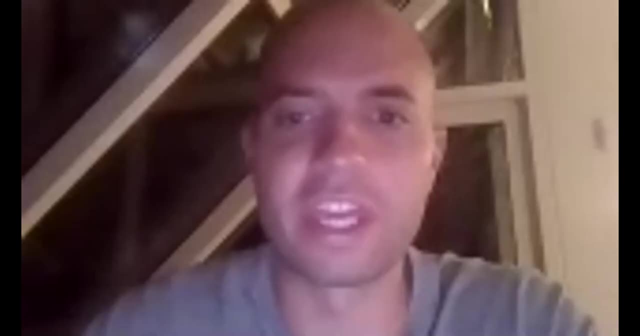 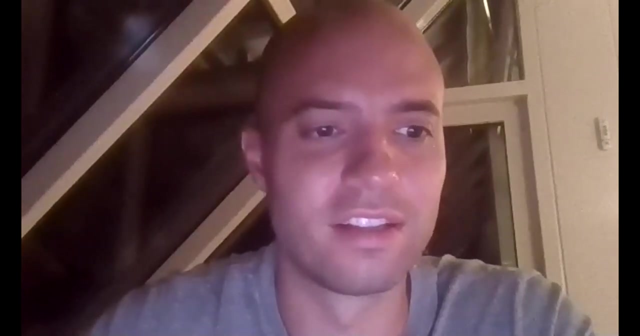 Pretty significant in your, in your experience. I'm not sure which part of the robot he's talking about. I think it's the last link that he mentions, the tibia link, the curve of the tibia link. I'm sorry, I didn't get what your question is. 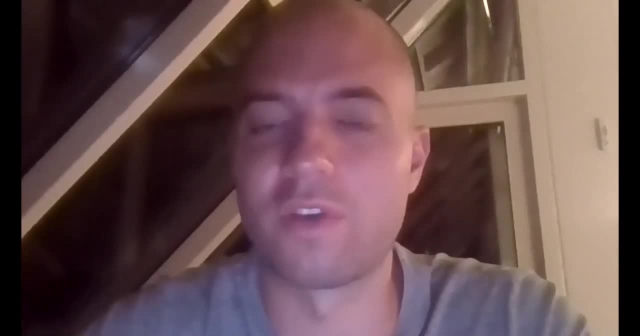 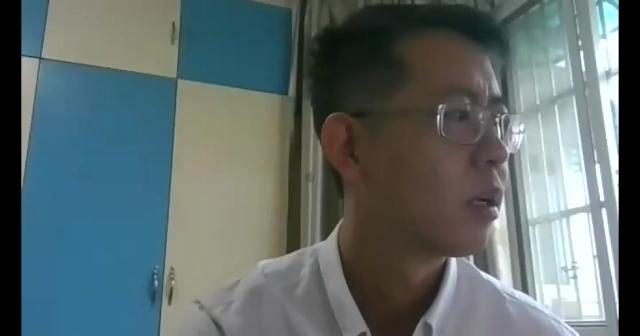 I think the question is regarding the last link of your quadrupedal robot, Last link That has a curve- Okay, And what are the advantages of that structure rather than straight, And what your advantages are regarding that Last link? 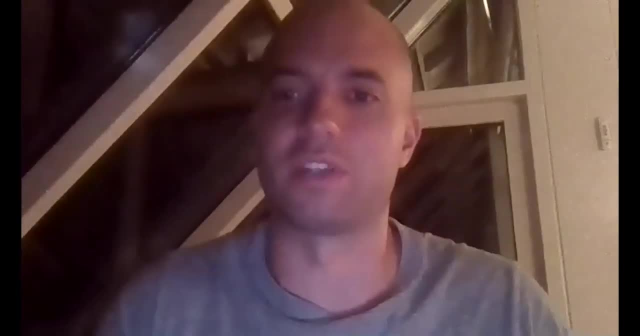 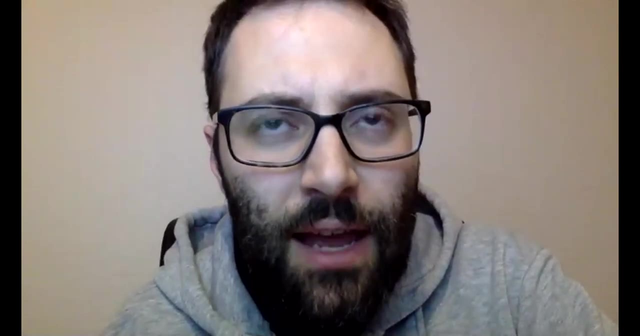 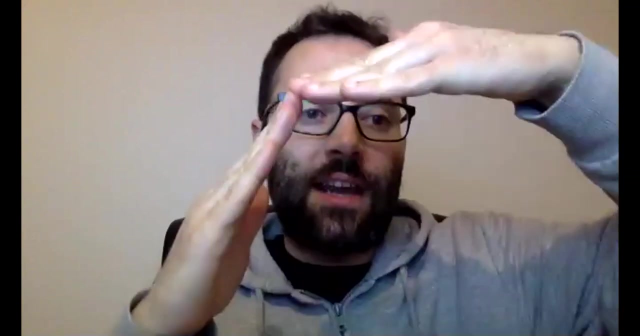 Yeah, it's, it's a curved link rather than a straight body. What are the reasons for that? Yes, basically why in the legs, the, the last link is more curved rather than, you know, straight links of the of the other quadruples it. does this give you an? 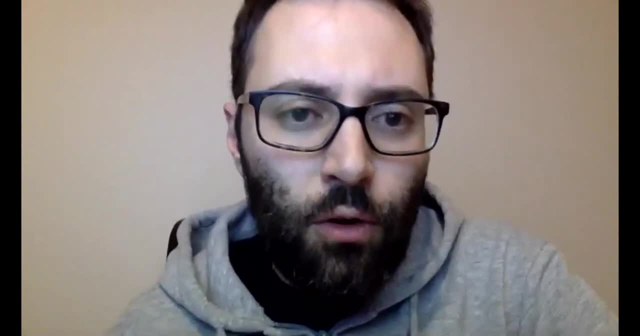 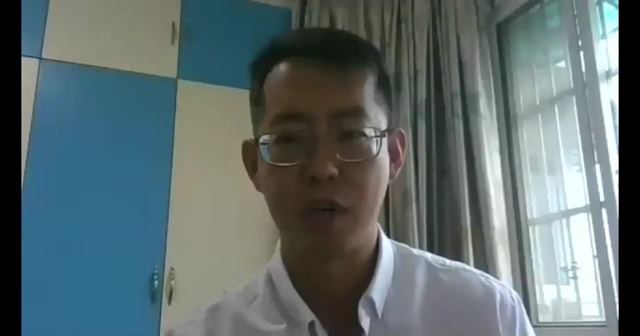 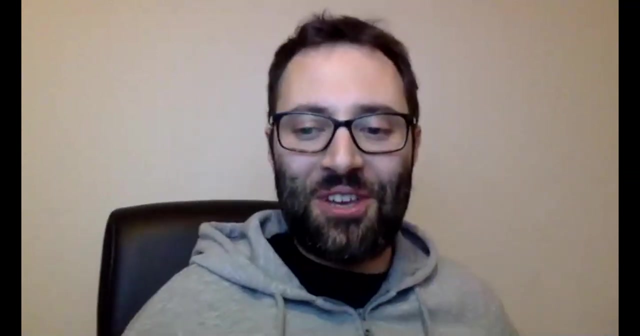 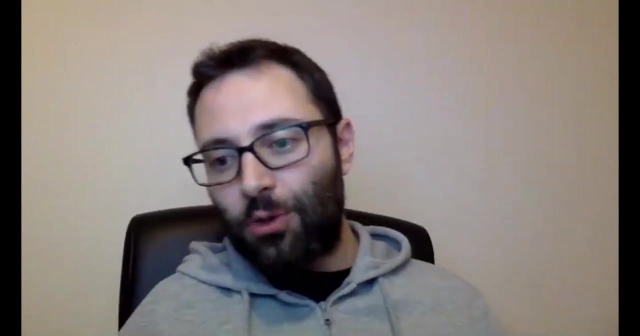 advantage on on the locomotion. I'm sorry I didn't do this part of a job because this was developed by another colleague. all right, so this is a more mechanical line equation. okay, all right. okay, all right, and I think, let me see. oh, I do have two, two last questions. one is so when, when we talk about this inspection, 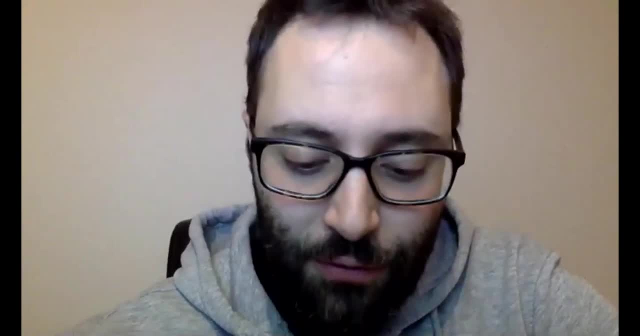 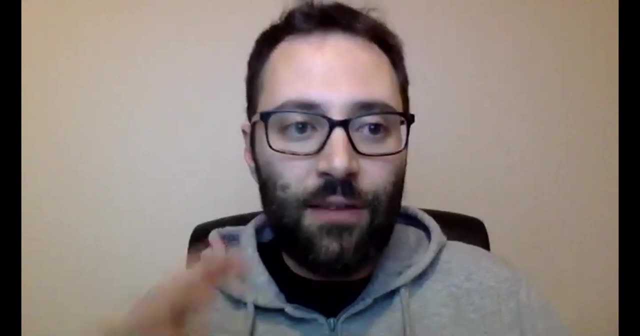 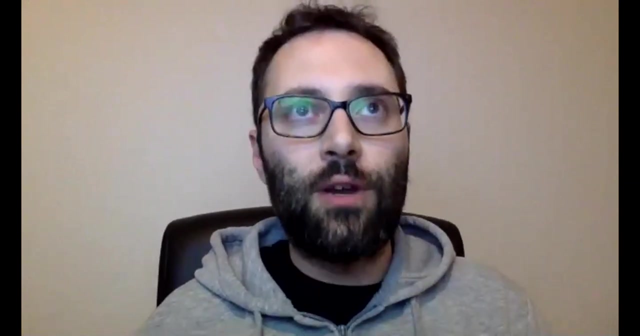 job. there is an interesting idea of you know, when you have to convince people to use robots over, just you know, several cameras around the building. so you know, my question is: do you see an advantage of really having a robot that you know goes around some buildings, rather than putting some just fixed cameras? 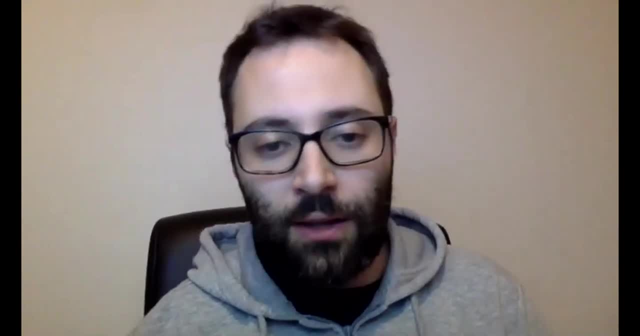 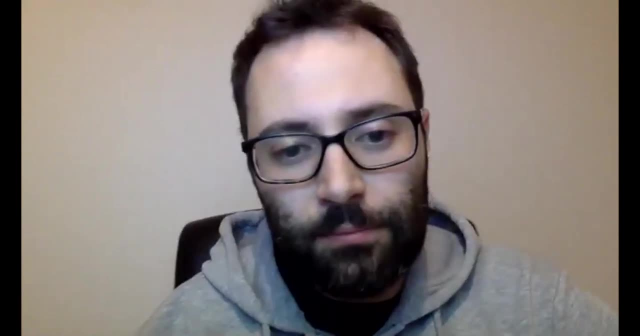 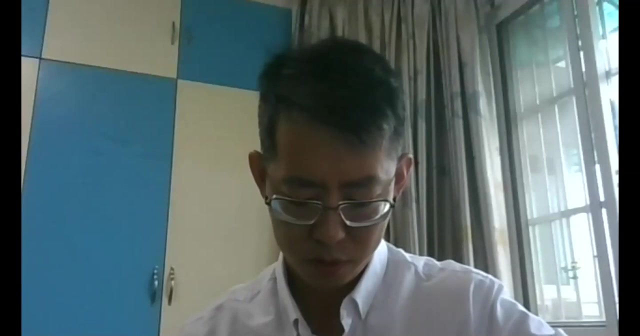 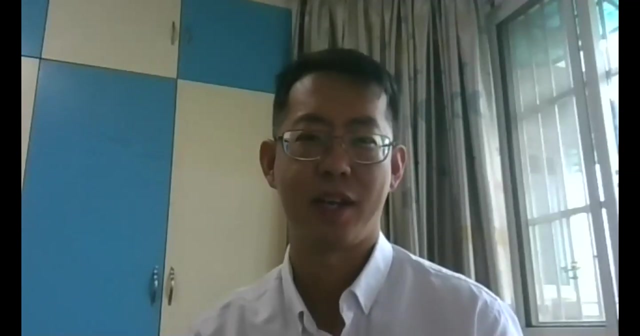 and then running something- inspection- with fixed cameras. do you see some advantage? is it more? make things more general, maybe? or yeah, that's a good question. and when we use a robot working around a building and with the cameras, if you can add a camera in the fixed position, it's definitely can be a good. 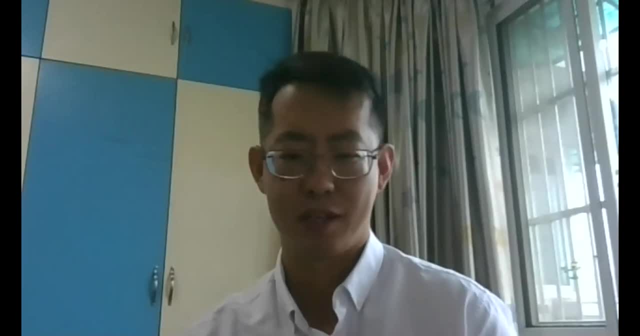 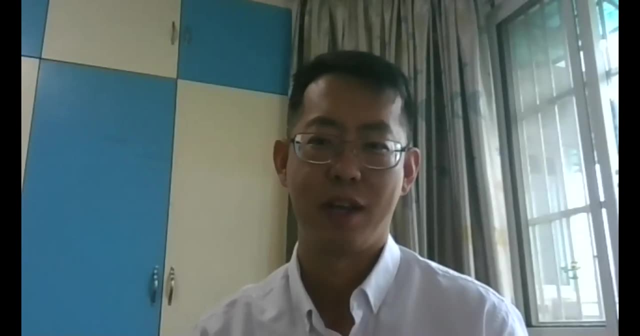 choice, but you have to think about it: the robot with the camera. it's like a. it's like a human takes a camera and the robot. you can save a lot of cameras because when you use a fixed position camera, you some, many, many of the places you want to, you want to monitor, right, if you have a robot with a camera on it, you can use a robot to. 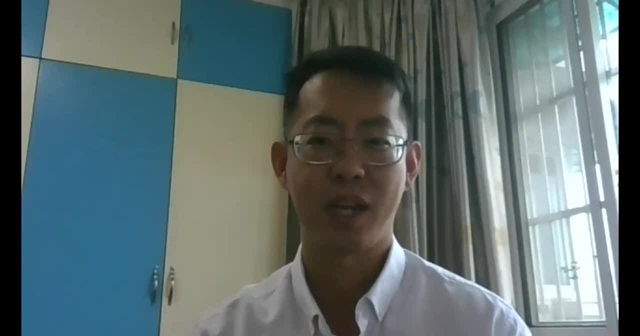 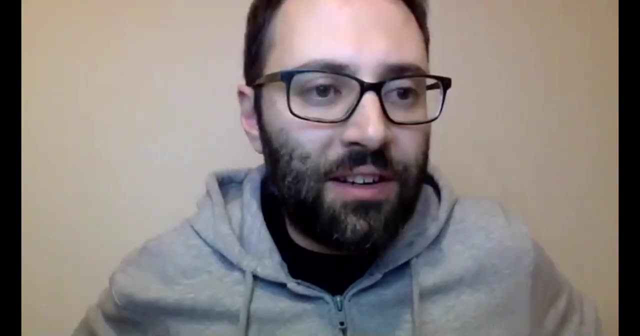 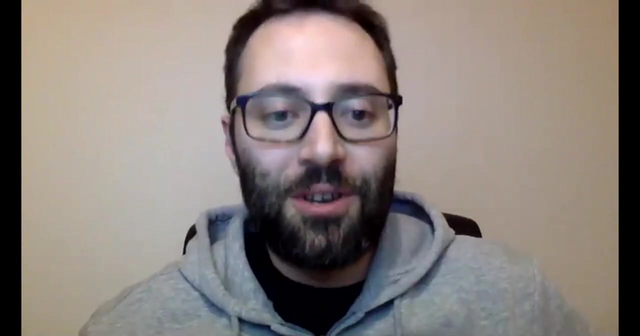 travel around and you just use one dog and then one camera, you can cover all the places that in your building, right? i do agree. i mean it's, it's, and i guess, like with inspection, it goes also the question of maintenance. so you know like at some point you will not only need to. 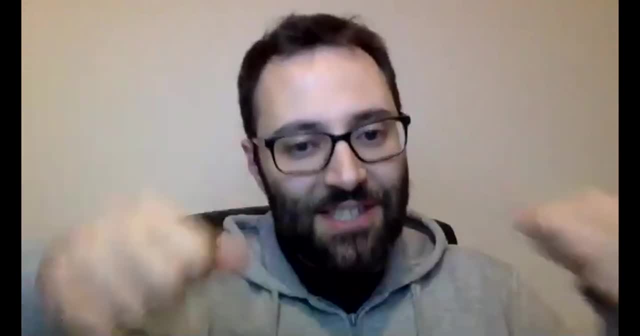 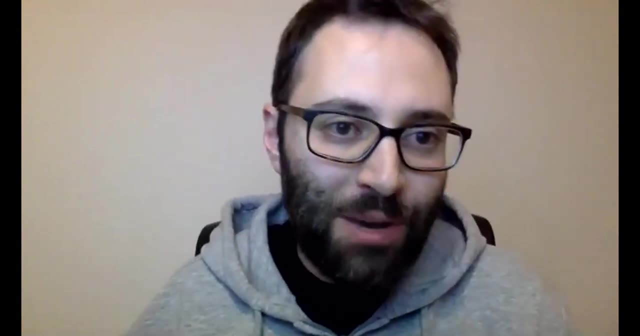 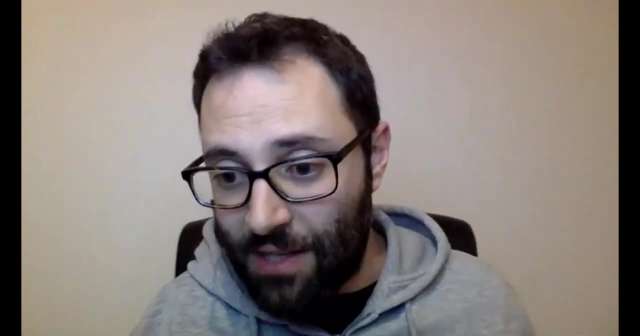 inspect things, but you know you need to. you know touch some things or you know like have a physical contact with some structures that you know a camera cannot do it by itself, so you need somebody, a robot or a human, to make this contact all right. okay, and the last question from my side is. this is regarding the last 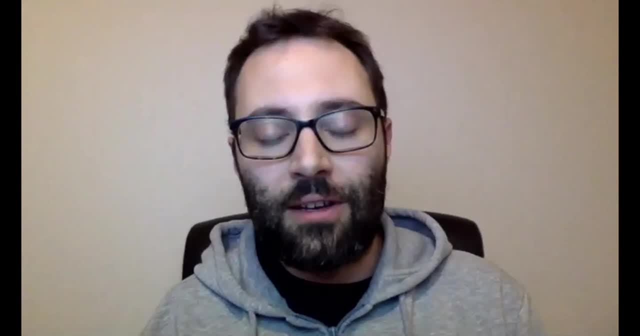 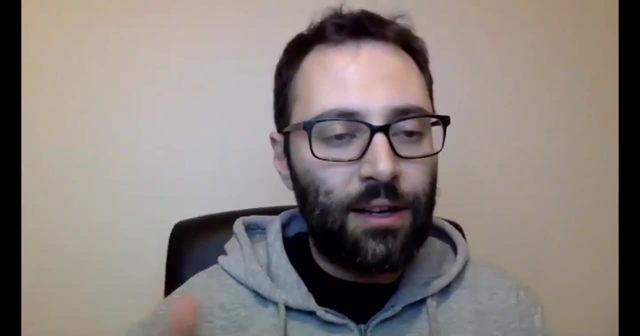 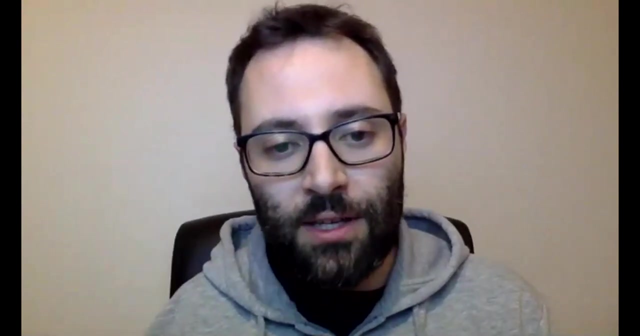 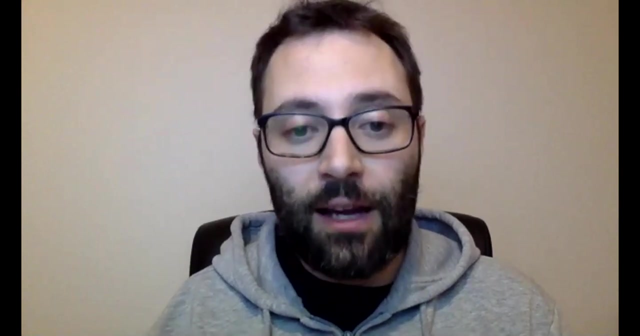 slides about the, the simulated environment. do you see any difficulty on training the reinforcement learning network in simulation? i don't know which simulator you are using. how do you apply this on there on the real robot? is it an easy simulation to real control transferability, or you train directly on the robot? okay, okay, this running. 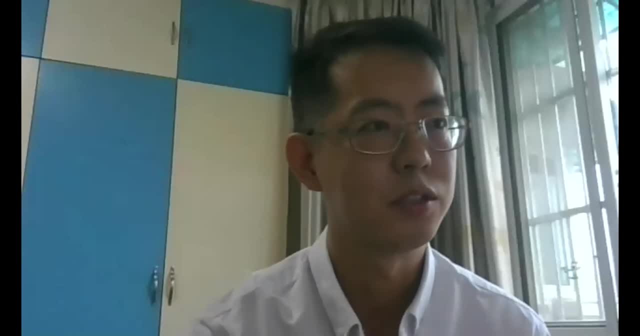 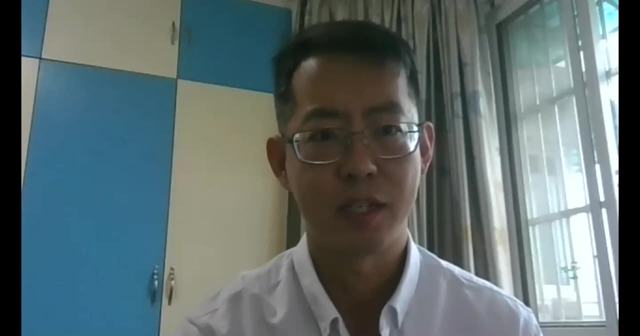 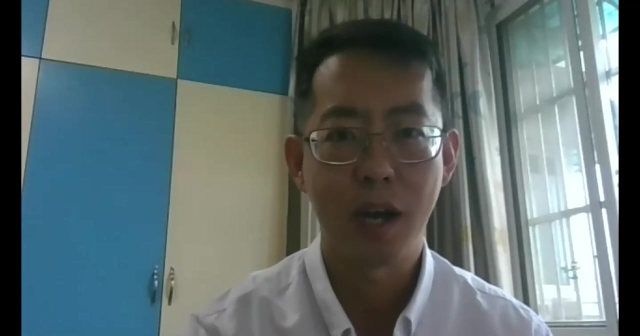 simulations. we we didn't apply the control theory in our real robot and but we have some cooperation project with other universities and when they, when they do something about the standing up with the reinforcement learning and we have tested on our real robot, but uh, the the papers over there is not uh published. 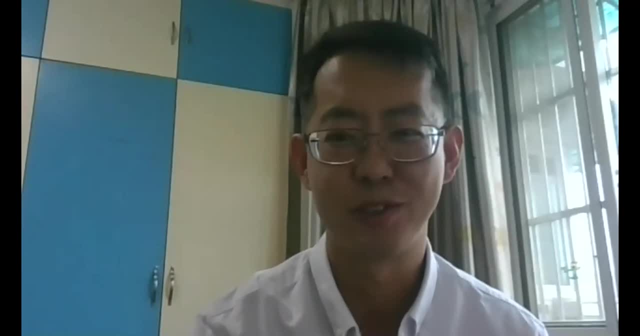 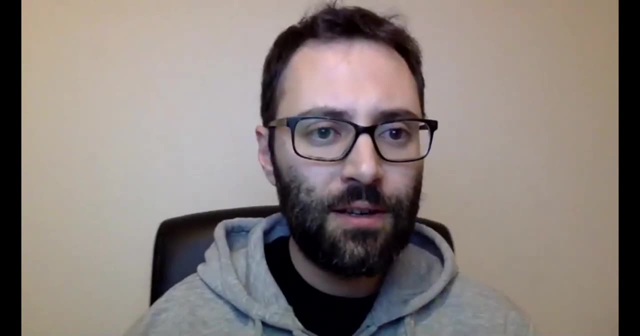 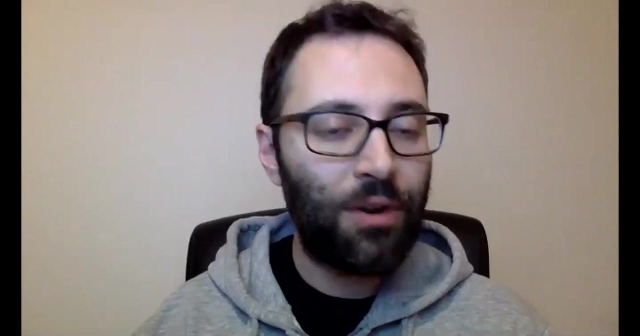 yet. so all right, if it's not good to show the videos to you guys, all right, okay, sounds reasonable, all right. so from my side, that's it, marco. do we have anything else? uh, for my, uh, wait. from my side, it's also good, all right, okay, thank you. thank you a lot for this talk.